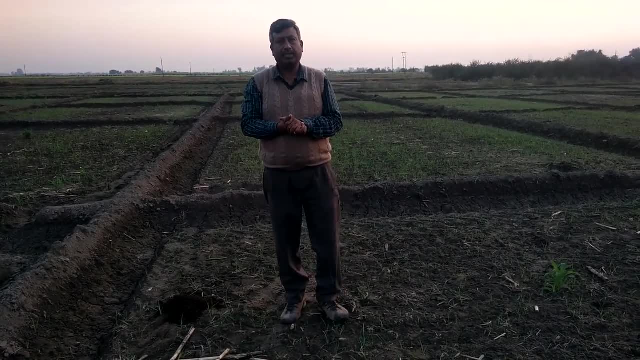 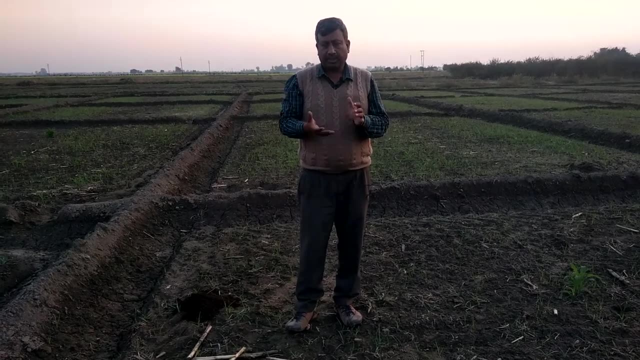 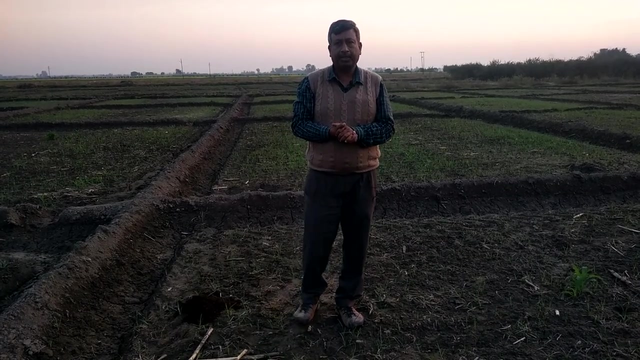 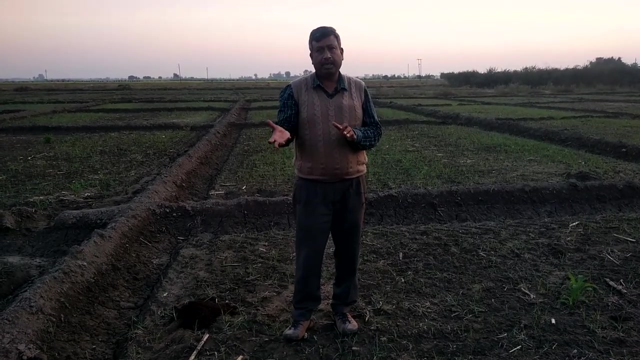 plant origin, So the organic matter that comes in our natural soil, that is contributed by falling leaf, So the organic matter is a leaf, So it is a plant which is rich in organic matter. and roots. So roots is the global source of organic matter and that's why the plant source is. 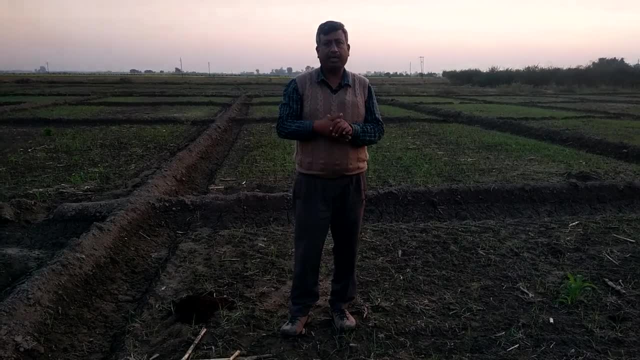 a major source and it is considered as primary source of organic matter. Then secondary source is animal and animal use. the this plant material, leaf, etc. and contribute as a waste urine or dung And after the death, their body also contribute in organic matter. that's why this: 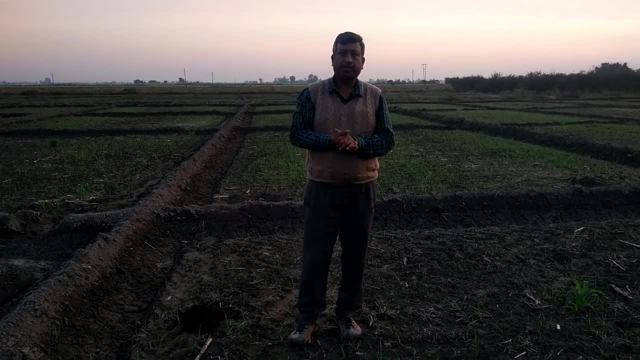 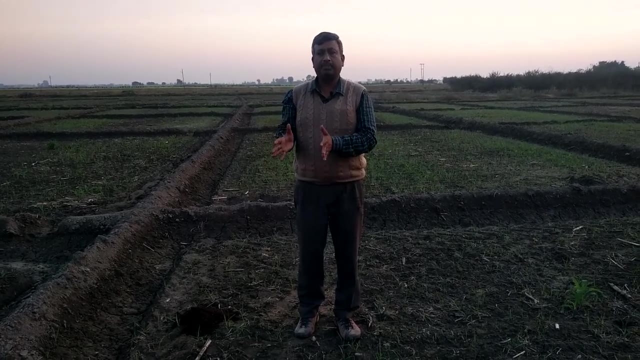 animal are considered as good organic matter And that is why the plant nature is so significant secondary source. so primary source plant and secondary source animal. to yet a plant products and China plant Cahoot animal, Cahoot jitra, be to contribute correct soil man that come under organic matter and after the addition of foreign 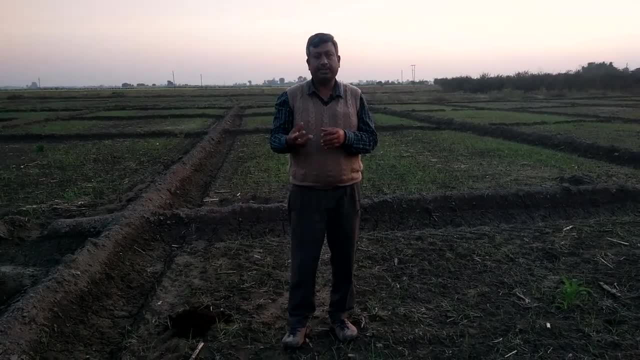 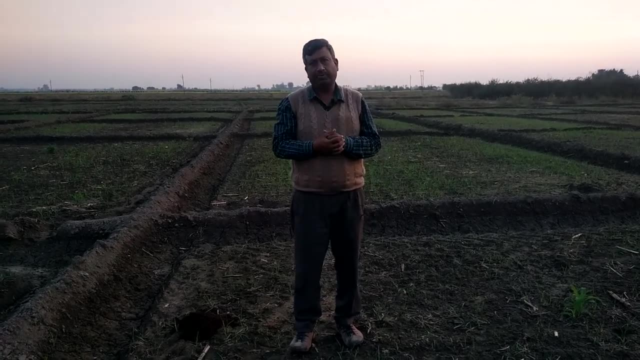 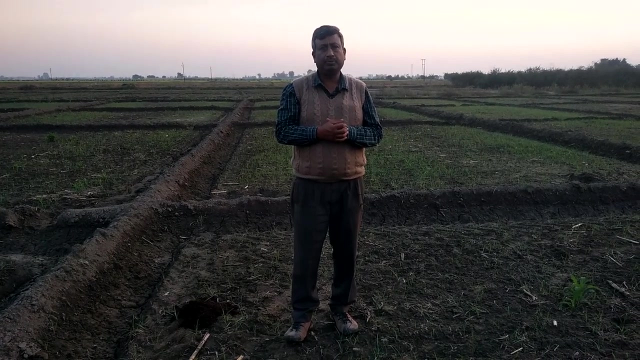 matter. when it is present, leaf or root or any animal product, it is undergo decomposition by microbes, bacteria, fungus, actinomycetes. so many microbes attack on this organ matter because they drive carbon as a food source and after decomposition, several nutrients are released. there is cities of a reaction. 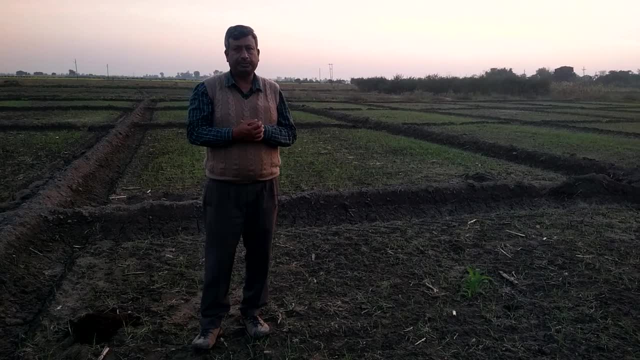 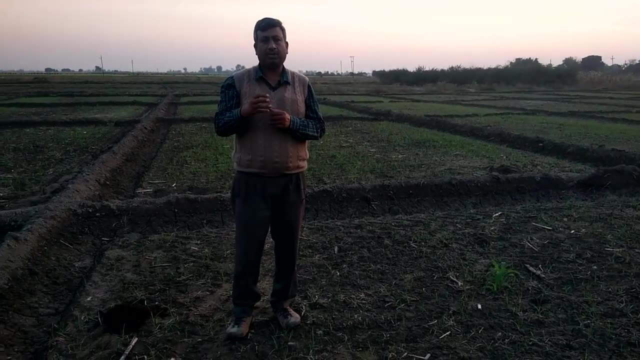 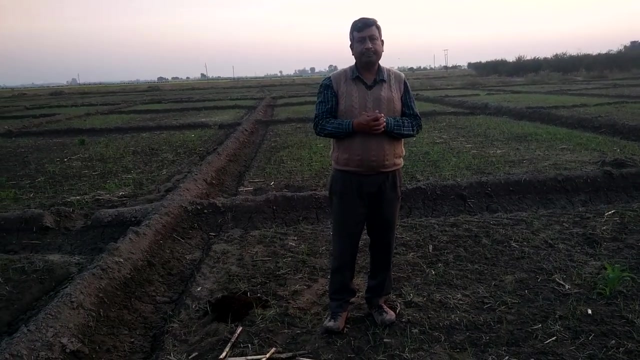 this is biochemical reaction and new compound synthesized and after the death of this bacteria, new compounds are there and another type of bacteria or fungus or other type of microbes attack further on this. newly formed compounds and another type of compounds are formed and after the back of such 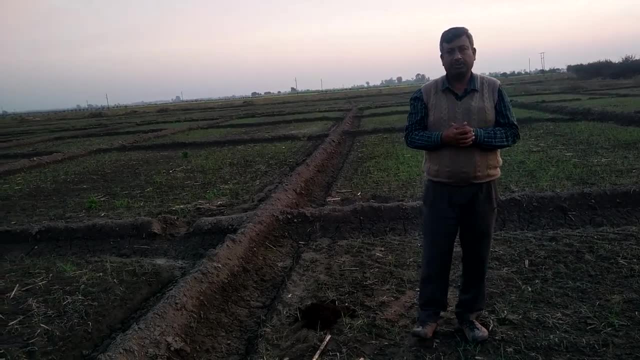 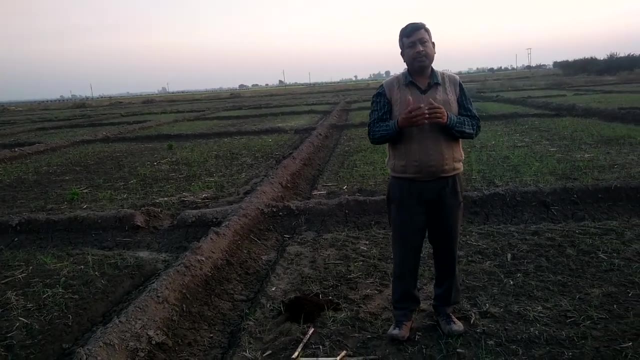 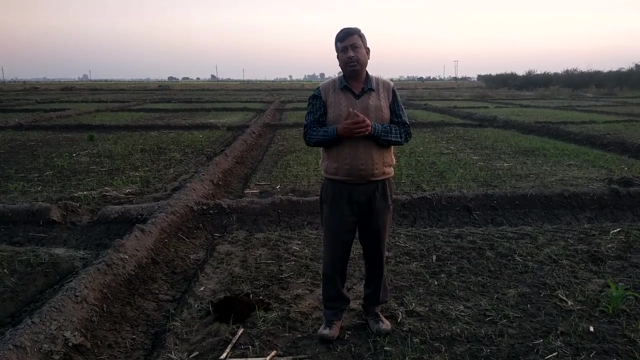 type of microbes. another third type of category of microbes is there and attack on this newly compound. So there is a continuous process of decomposition and new compound formation. and this new compound formation take place in microbial cell. so decomposition will happen and newly compound are synthesized, and after that, when this series will go on, then there is a polymerization. 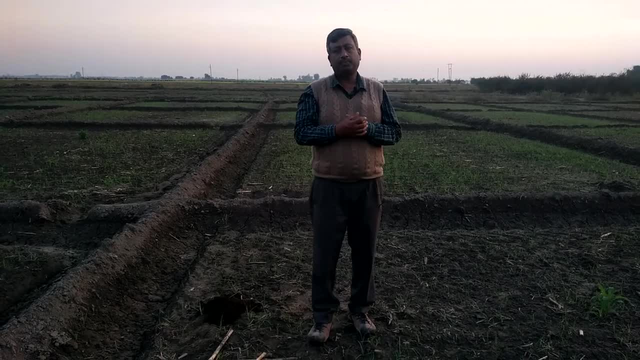 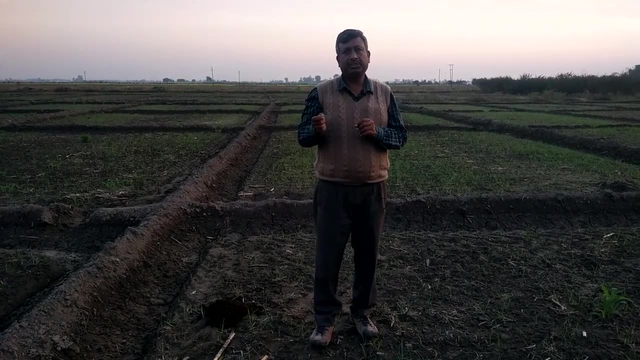 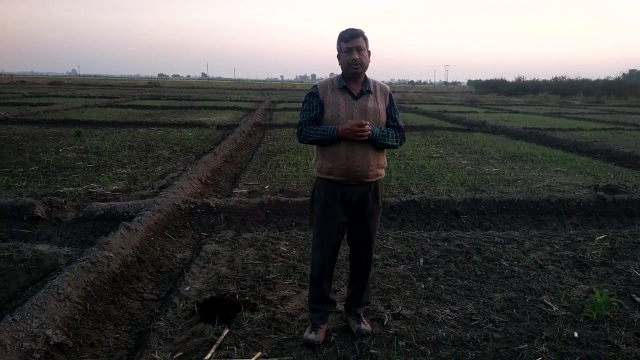 of compounds. so there will be a polymerization, new compounds will be made, and this is a complete series: decomposition, synthesis and polymerization. and now there is a condition that now this newly formed substance is not subjected to decomposition. now it is resistant to decomposition. 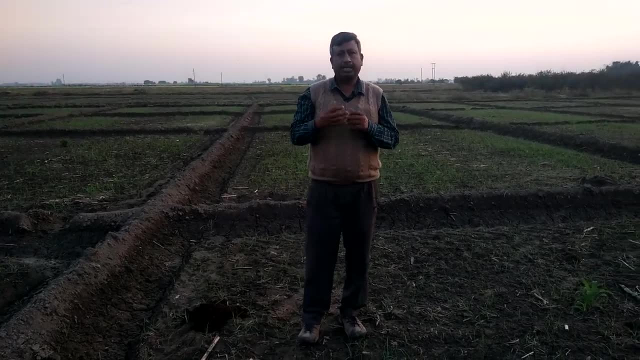 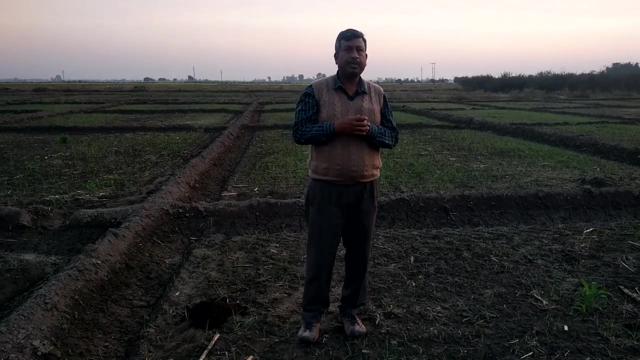 because it will become so complex that further decomposition will not be possible. and this newly formed compound, or we can say that is the complex compound, is termed as humus. so this is humus, from where this is made. This is the decomposition of the organometer. 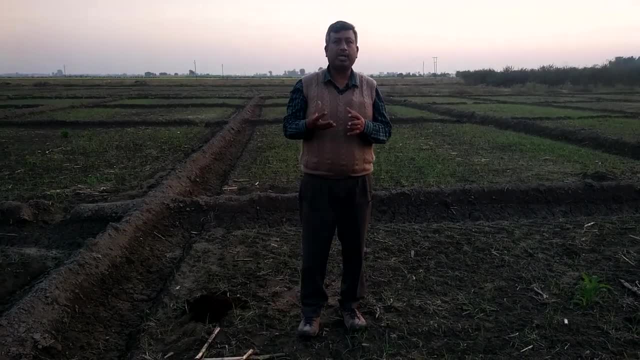 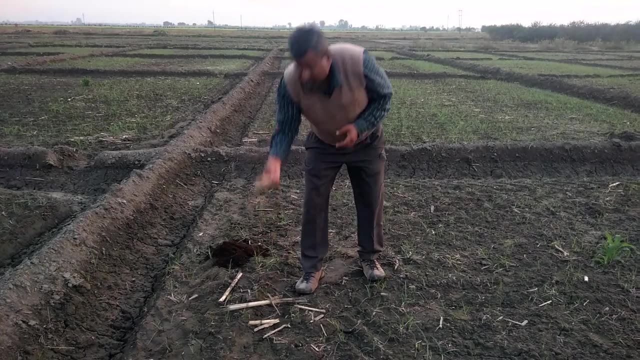 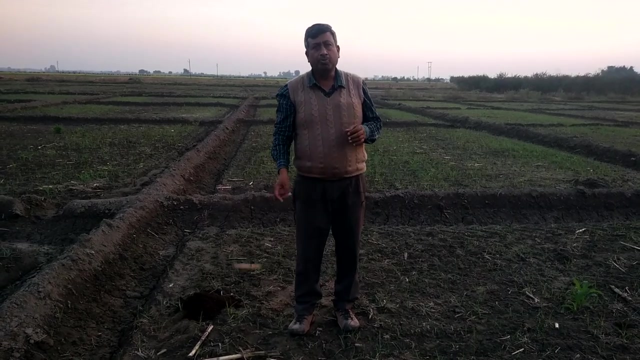 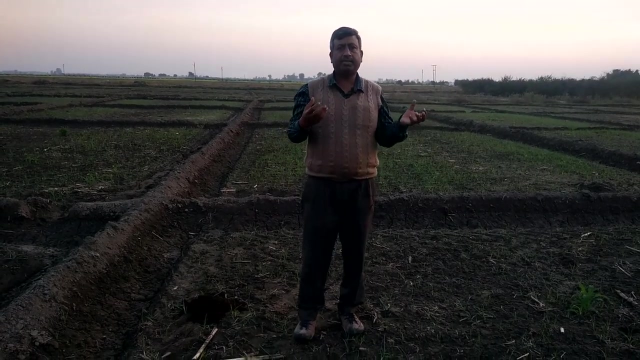 This is a newly synthesized compound and polymerization happens. So what happens in humus? there will be a lot of new compounds. there will be a different type of compounds that were not there in the original, which are in this type of plant, which were the residues or dung or urine, which has compounds, which will all change. 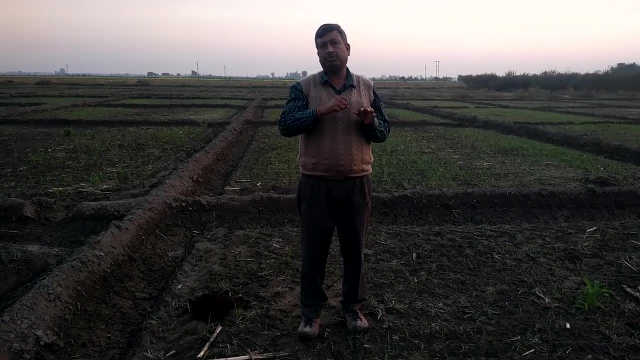 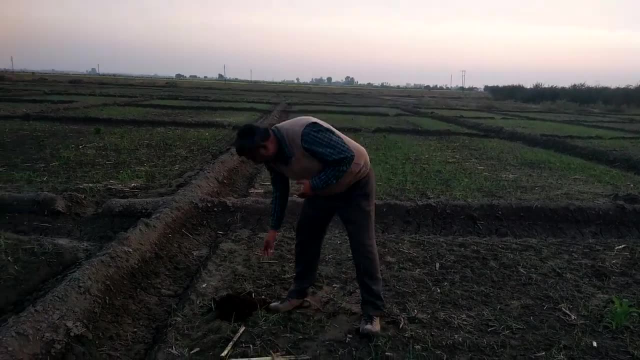 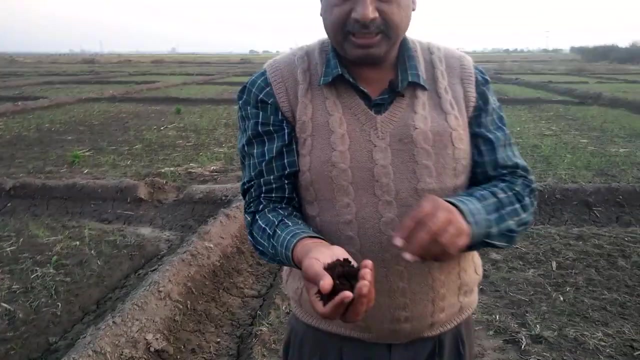 in a complex compound, and that will be called humus. Now, humus is completely a different substance. New compounds have been synthesized, polymerization has been done and many compounds have been made. If you look at this, you can see that this soil has been made after the sowing of cow dung. 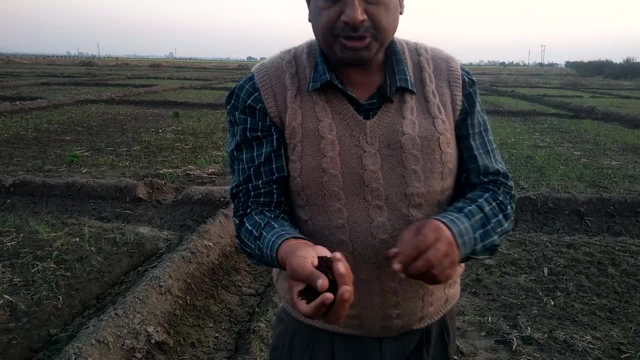 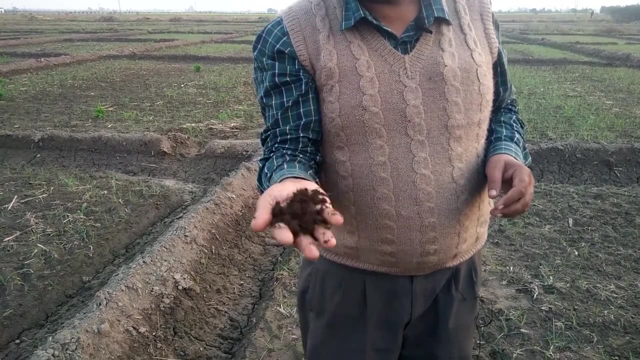 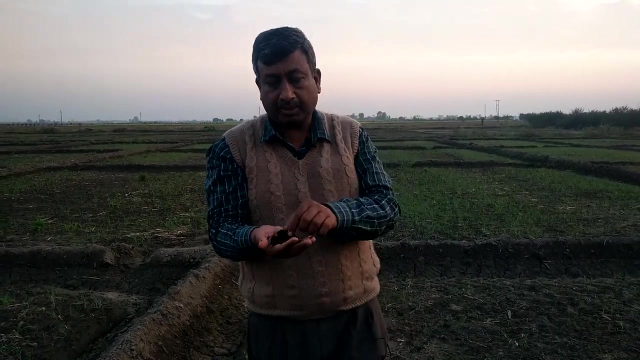 What kind of changes have been made to it? It has decomposed completely and it is very light weight. it has become dark brown in color and now it will not decompose much Because after decomposing a lot of compounds in it, such compounds have been formed that further. the microbes will not attack it and they will not be able to take carbon from it, because the carbon chain has become very complex. 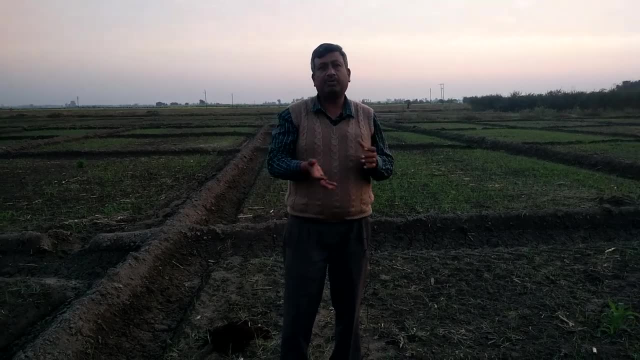 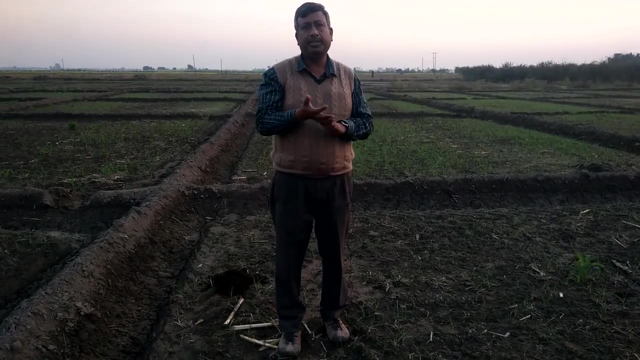 Actually, what happens is that the microbes decompose for carbon and for nutrients, and when such a series of compounds is formed of very complex compounds, then the carbon chain cannot break from it. So the same compound that is made in the body is made of humus. 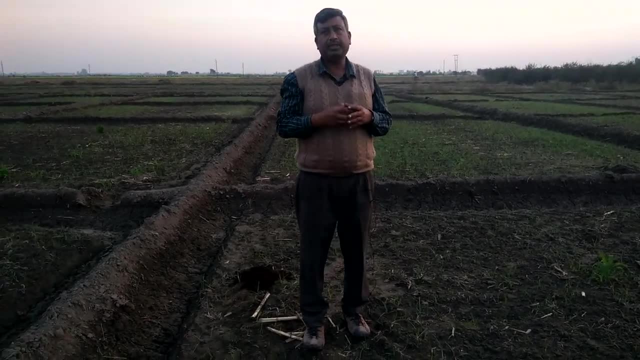 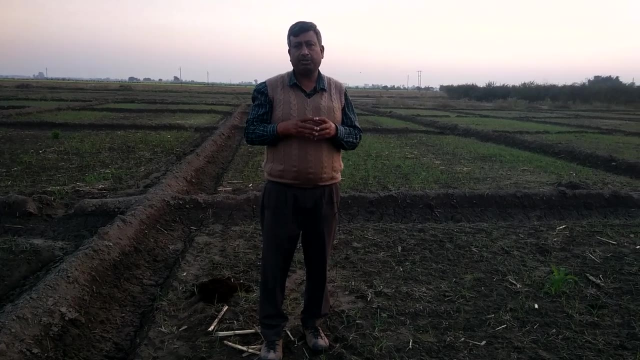 So the nature or process of humus is very interesting. It is a complex process and it is not fully understood yet and its very precise mechanism is not very clear and its nature, how it is made, which compounds have come. its knowledge is also incomplete in the whole process. 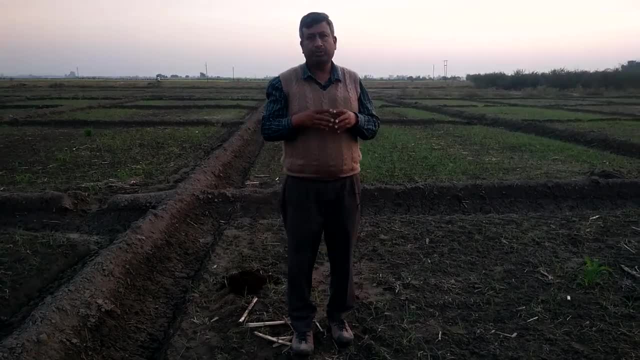 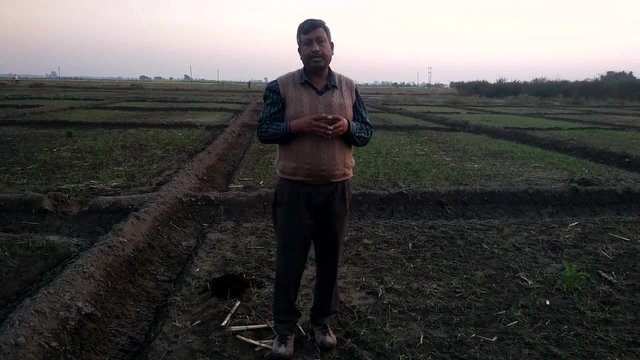 Now research is going on on how it is being processed. So humus is a very complex compound. So if we look at its definition, then it is a colloidal compound. It is colloidal, fairly stable- Stable is being said because its further decomposition is not happening. 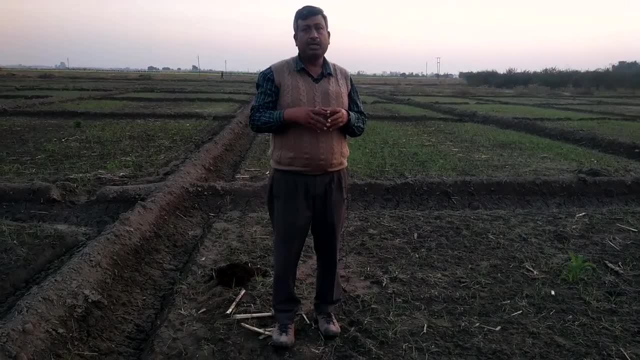 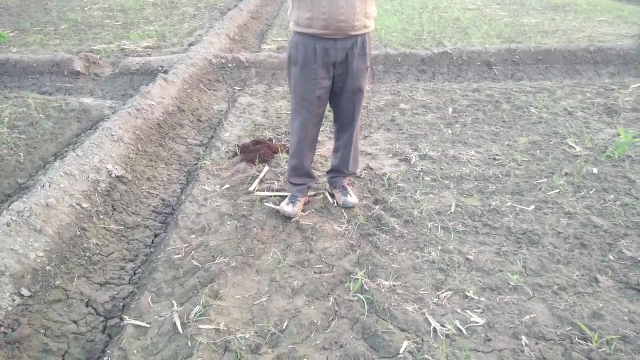 Amorphous: there is no particular structure in it. Amorphous: there is no particular structure in it. Amorphous. dark to brown colour. as you can see, it is brown in colour And resistant to decomposition, and further decomposition is not happening. 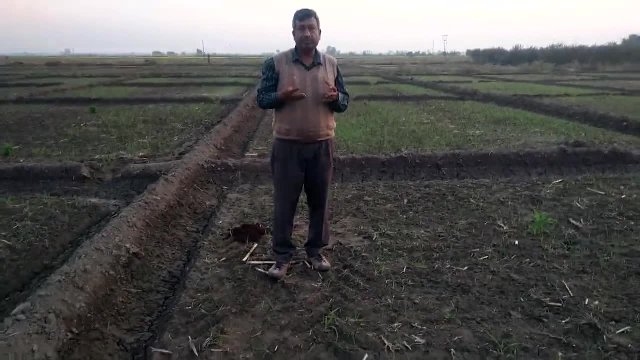 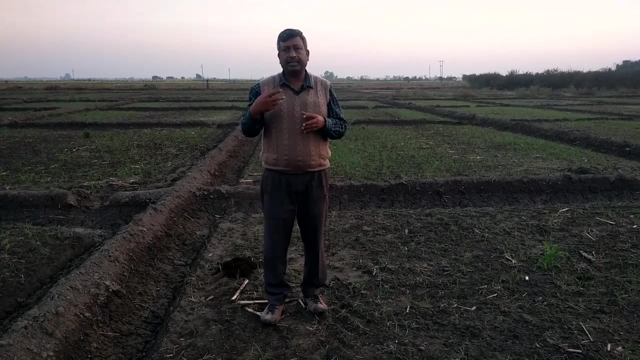 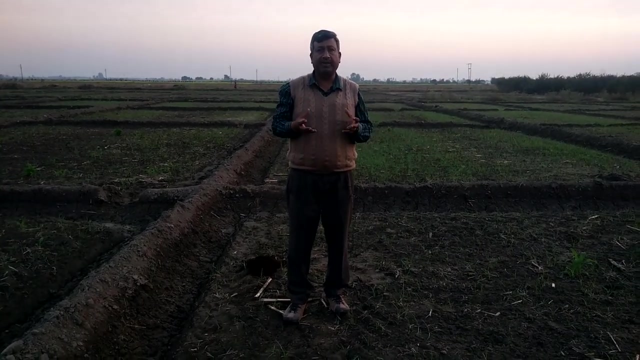 This is humus and this process of humus is known as humification. So this is how humus is made And the characteristics of humus. that characteristics affect or influence the soil properties And these are very favourable effects. There are very favourable or very positive effects on soil properties: physical properties, biological properties. 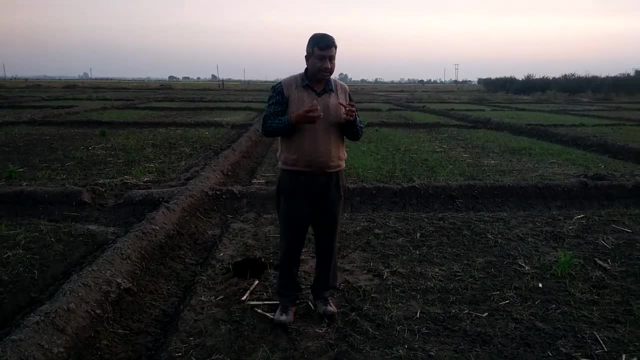 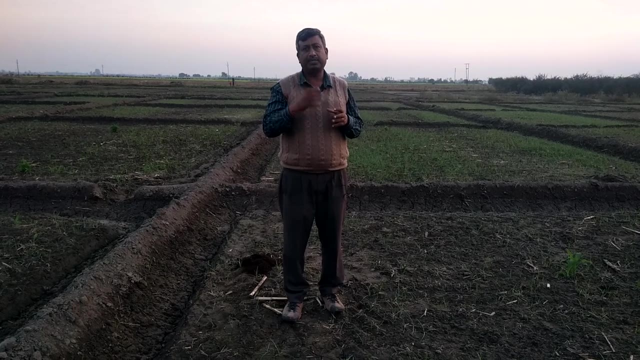 biological properties, chemical properties. We will discuss this. So let us first know the characteristics of humus. What are these characteristics? First, I told you that it is colloidal. There are very tiny particles, very minute particles. So it is colloidal. 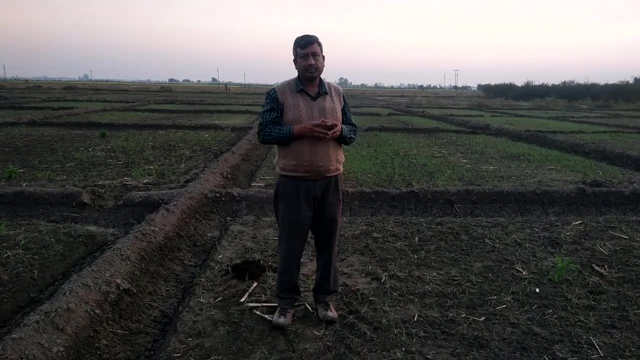 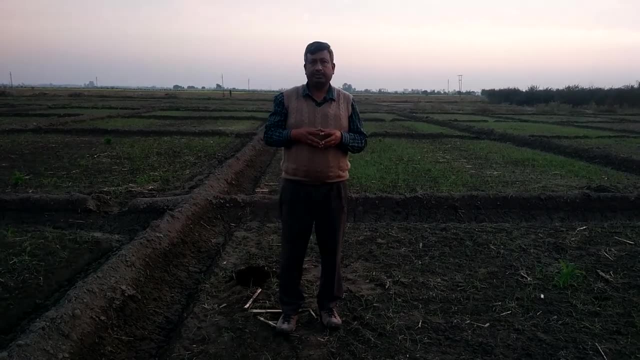 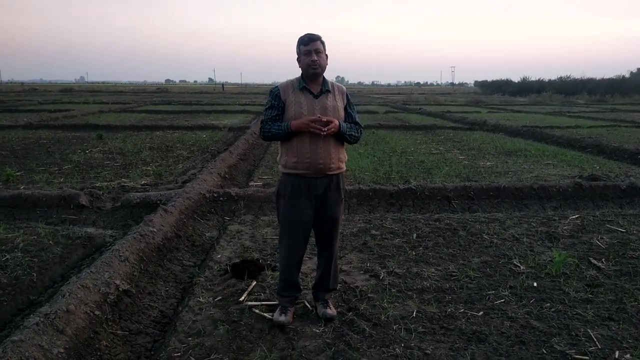 nature And because of this colloidal nature it has a very high surface area, high adsorption capacity for water and it has very low cohesion property, low plasticity. So this is a favourable fact that it has low plasticity and there will be no stickiness in it, And this is its 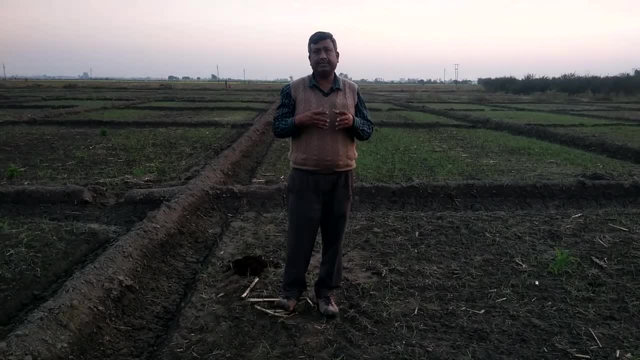 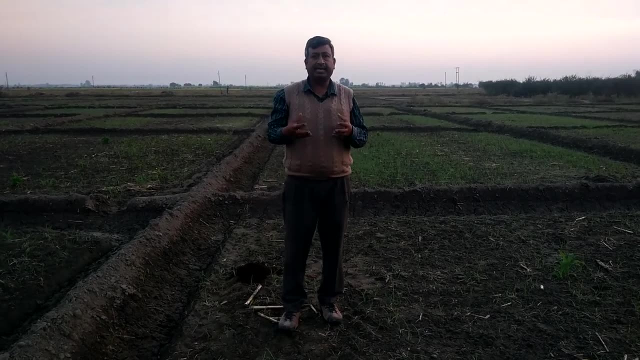 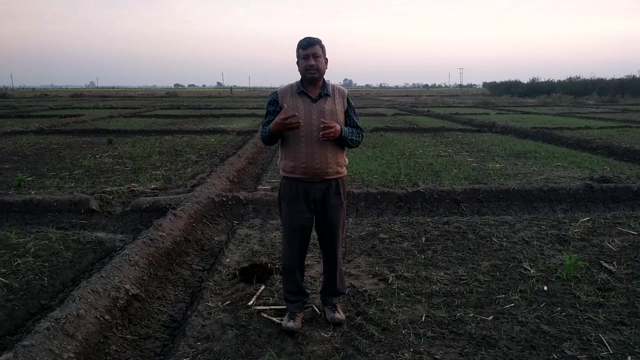 colloidal character and it has a high CEC catenic exchange capacity. Because there are several new compounds, polymerized compounds, and these compounds carry negative charges by hydroxy hydroxy group, OH group, carboxylic group, COOH group and phenol group, And these 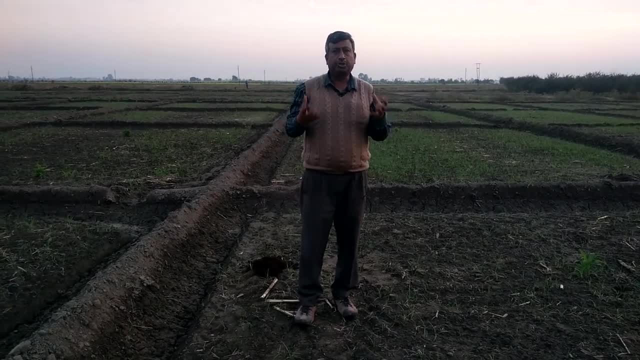 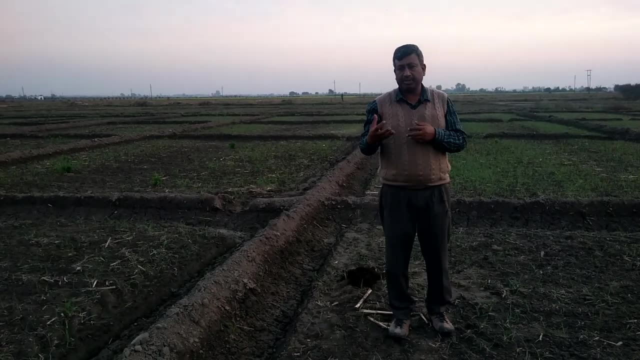 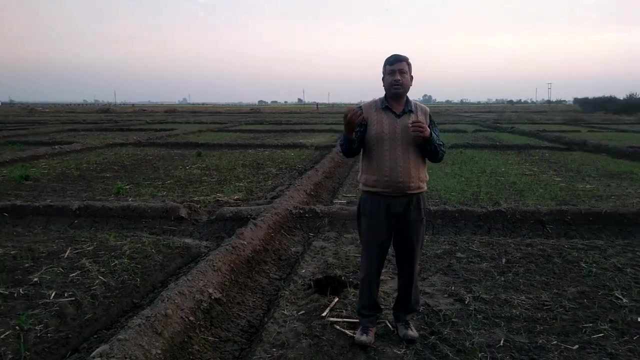 negative charges are very huge quantity and that is why they attract a lot of attention and attract the cations like potassium, calcium, magnesium, ammonium, And this cation exchange is similar as that occur in case of clay particle, So as there is a negative charge in clay, 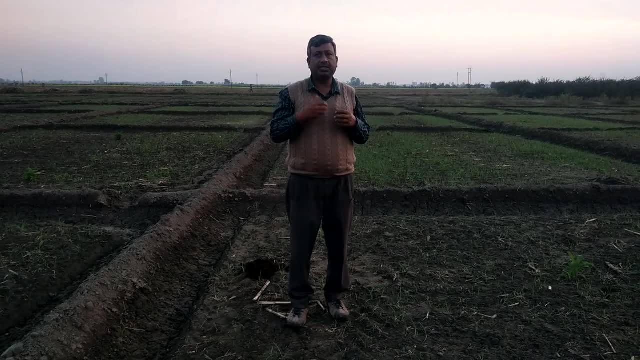 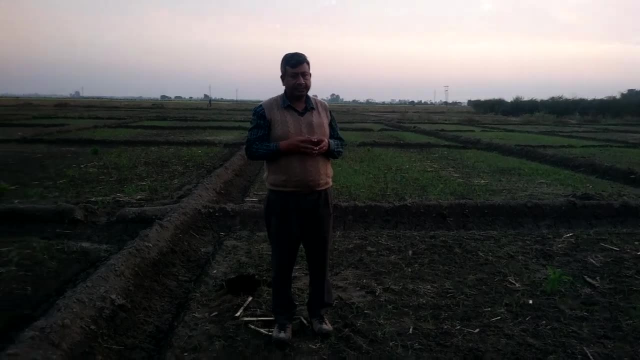 and it attracts the cation and then it exchanges it to the solution. Similar is the way in case of humus. So humus has high CEC and has negative charge and carry huge quantity of cations. So this is its very good character: that it can attract the cations. So this: 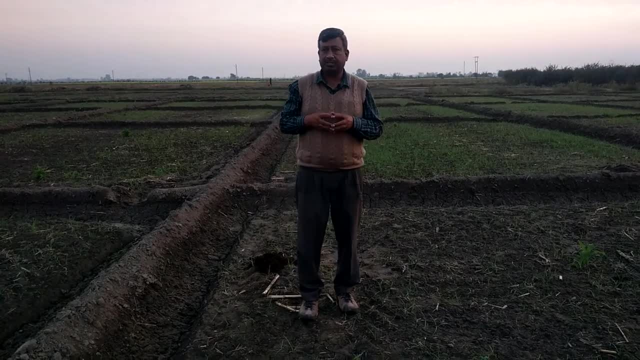 is its very good character that it can attract the cations. So this is its very good character that it can attract the cations. So this has very good characteristics and it has general particular in Ramira, which is similar to catenic CEC. 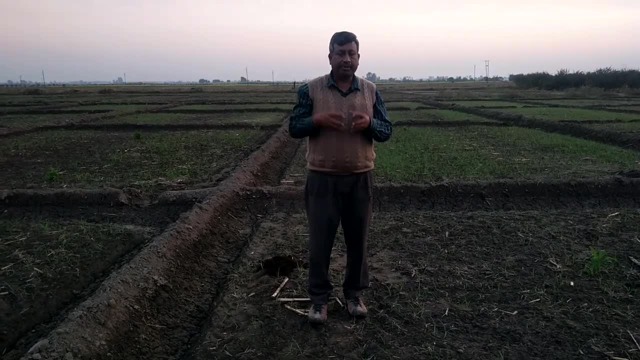 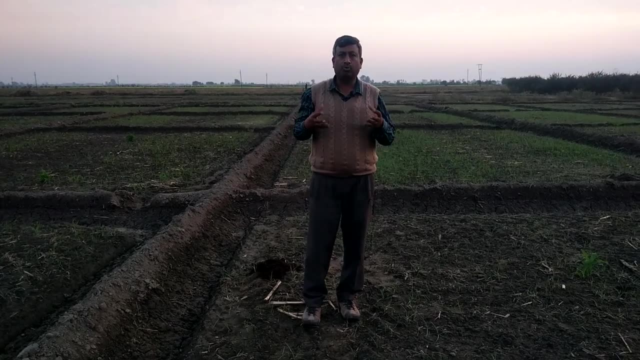 particular CEC. that well, So that means its active andoga itself. Otherwise its active andga is different. otherwise its active andga is different that you can get a low CEC setting in its state with high CEC and a low CEC. So Humus's properties have very strict category. 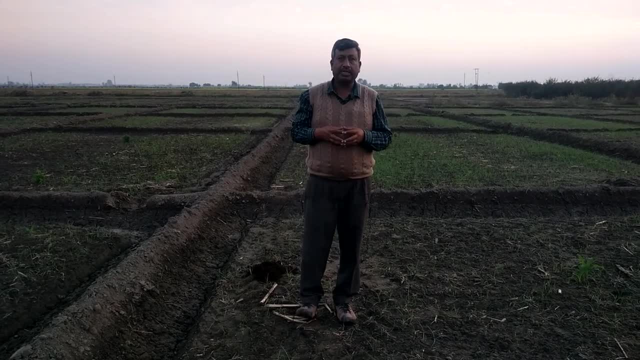 so through that it keeps some catenci to be. it has otoc yön Мы्е, not şimcy кор FeH неё, and is bring nearруж à puppy. dái delayed production too, And these zatigbe. 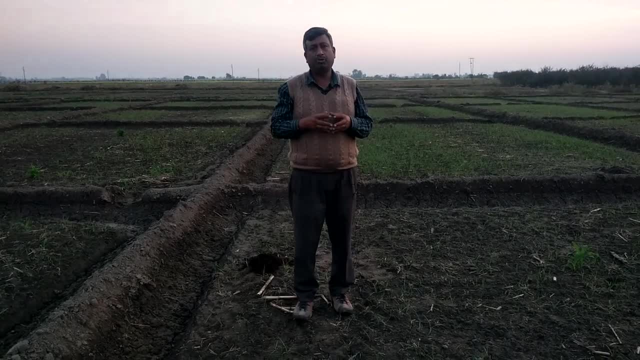 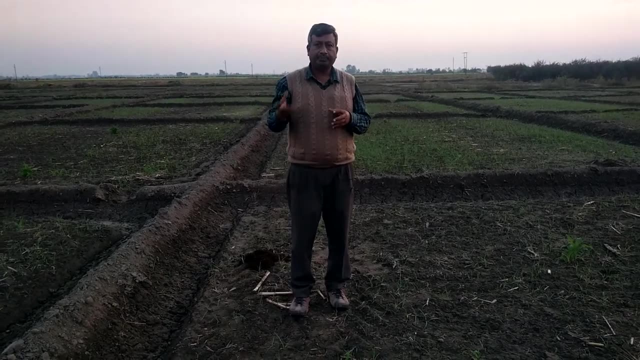 the cations below the roots? yes, because they have bacteria that can keep. Otherwise, if cations will leach from the soil and go below the latejewel, then it prevents leaching. highly resistant and these contain polysaccharides and polyuronides, and these polysaccharides are 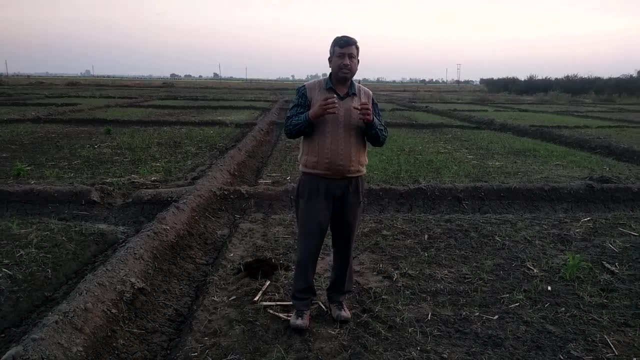 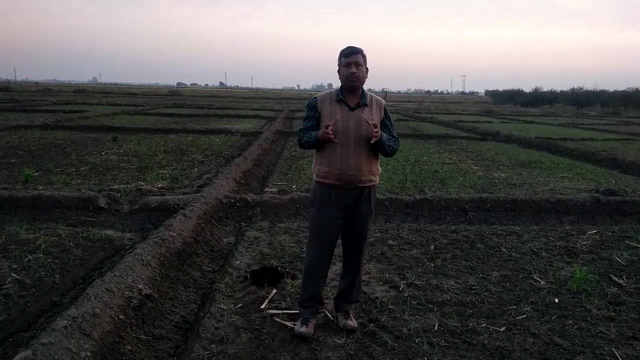 especially effective in soil aggregation, The aggregation of soil particles, which I have already explained in previous lectures. these are very highly helpful in soil aggregation. So there are two types of groups: humic group and non-humic group. Now we will tell you in detail what is found in 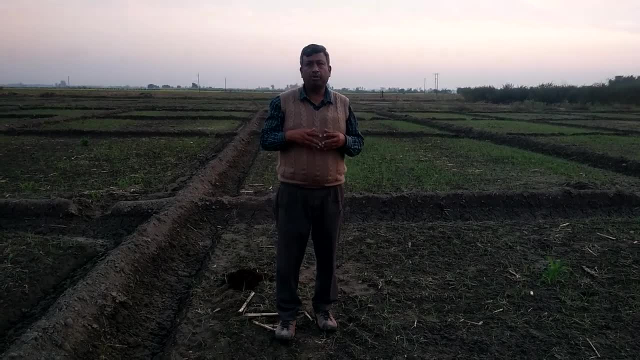 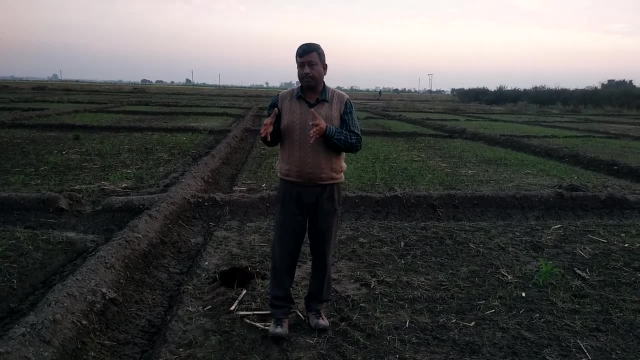 humic. There is filvic acid, humic acid and humin. The proportion of non-humic is very low: 20 to 30 percent, and 60 to 80 percent is humic group. So these types of compounds help. 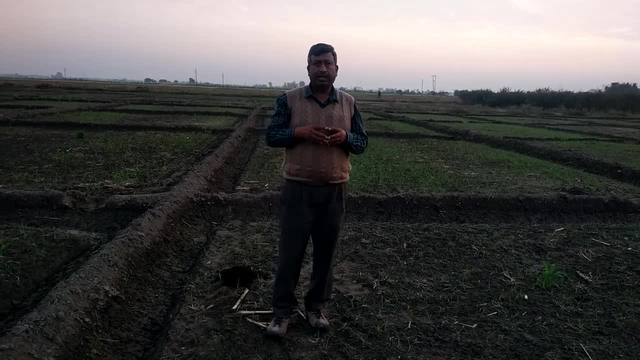 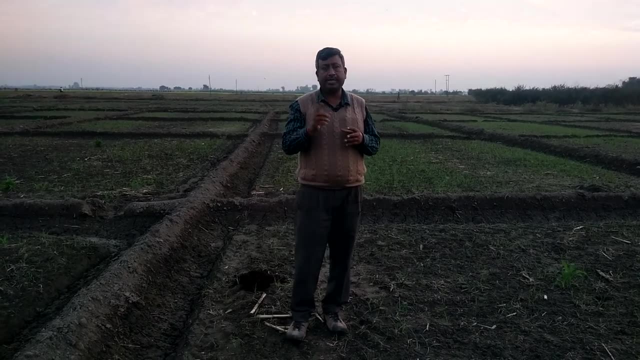 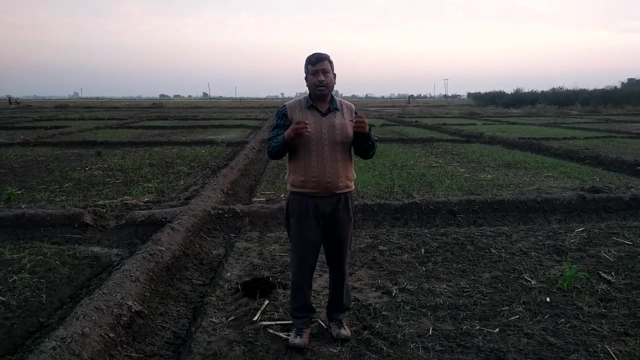 particularly polysaccharides, in soil aggregation and this humus make a surrounding or make a coating around the clay particles, So the coagulation of clay from electrolytes prevents. it acts as a glue, acts as a cementing agent and when this humus comes it helps in aggregation. 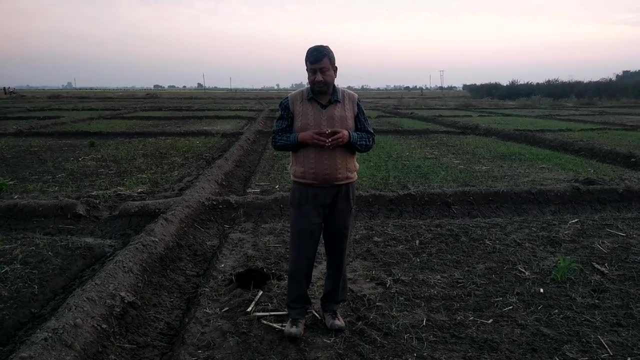 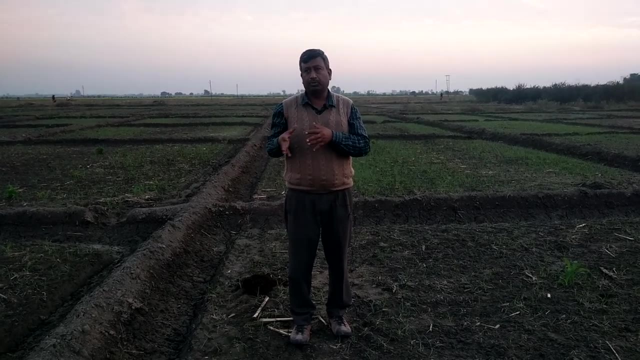 So it helps in the aggregation of clay in this way. and when there is a humus, definitely fungus is there and fungal hypes are more. and this fungal hypes help in aggregation also. So humus is helping in two types of aggregation: one by polysaccharides and 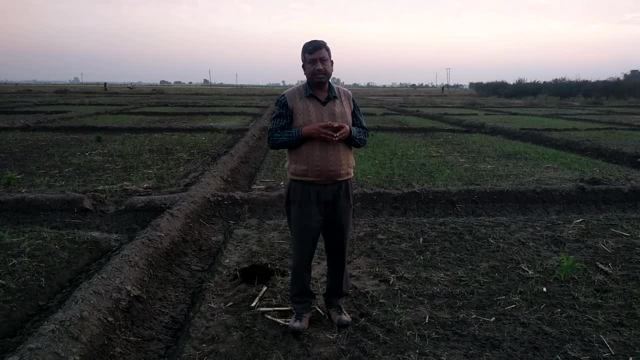 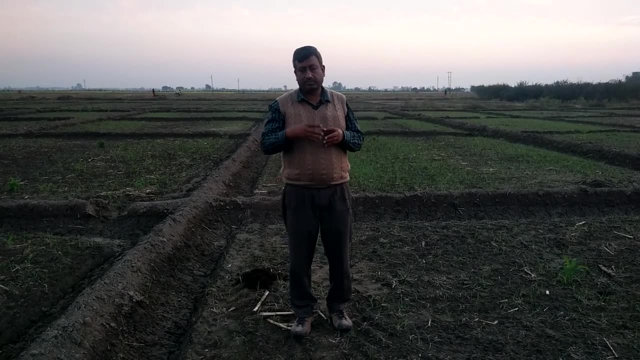 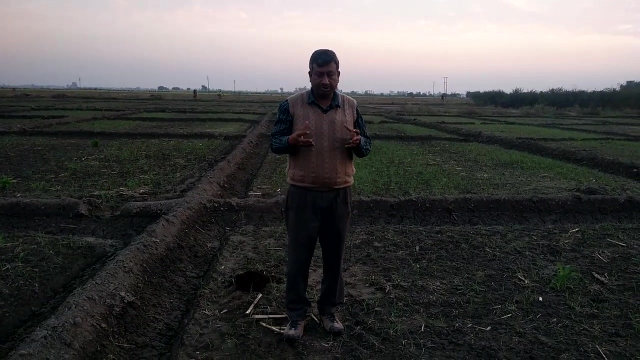 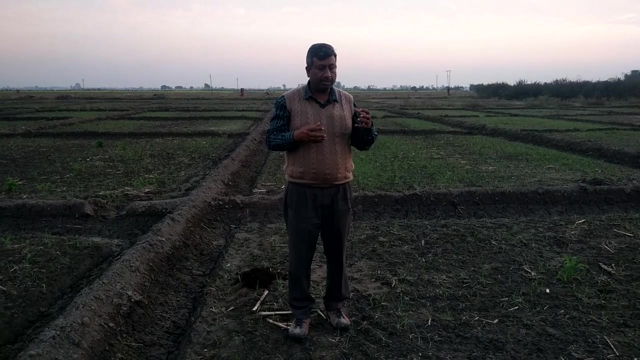 by fungal hypes. So this is one of its characteristics and, if we look at it in more detail, so it is holding the cations. in the same way, it reduces the toxicity of aluminum, the acidic soils and it reduces the Корinooth Similar to this. this organometal complex is made and this organometal 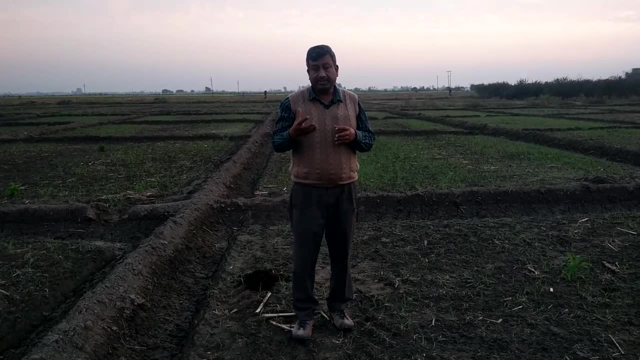 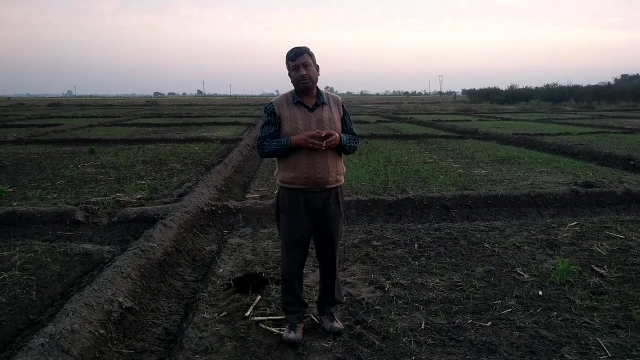 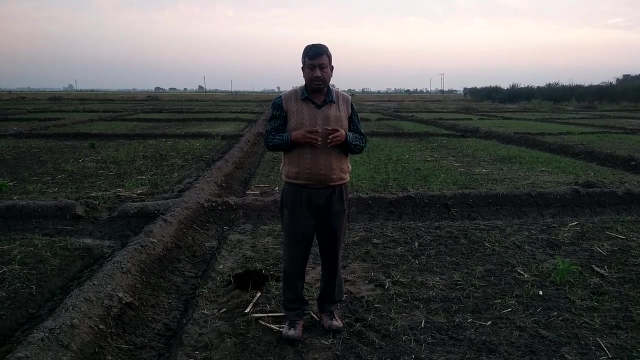 complex, is stable and will absorb polytains, also like lead, cadmium. So that is why helpful in reducing water pollution. otherwise, what will happen that cadmium and lead are in soil? then what will it do? it will leach and run in the water body and pollute the water body. But if there is a humus in soil and it attracts the resins which attract the and PVP. The cadmium and lead will not, Similar to this, release lead into the soil directly through catfish crystal, which, läng, does not cause corrosion to the soil. instead of there being a propulsion at that path, the cumin still acts as a constant. 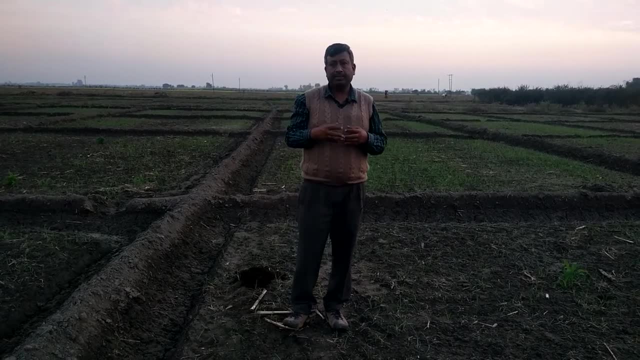 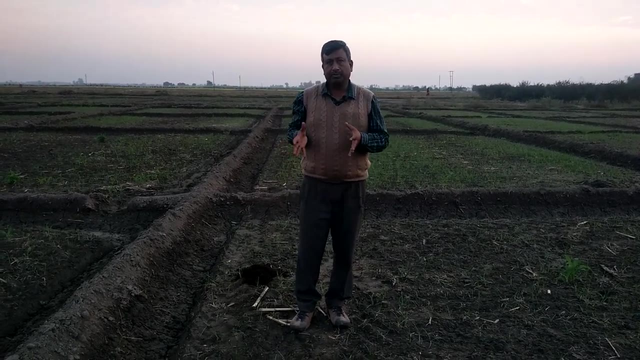 then we also have that squeeze in the soil. so if there is an oleic acid, then at that time make bond between the cation, like heavy metals, and thus prevent the leaching and there is no groundwater pollution. So this is what I told you about humus. 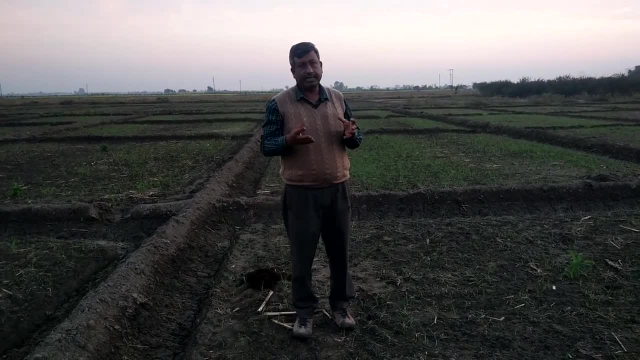 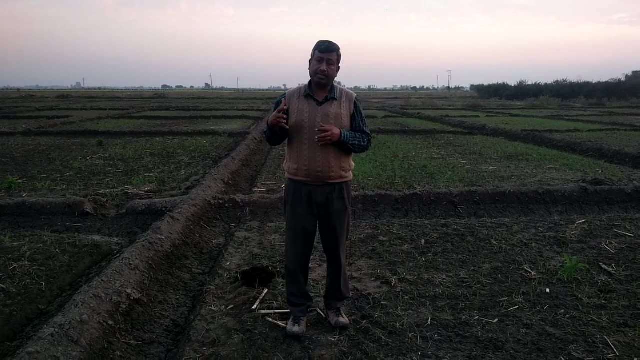 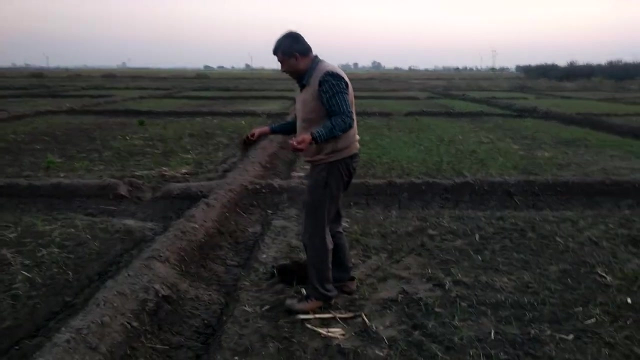 characteristics and its high surface area absorption capacity is very high. it is about four to five times higher than silicate clay, so four to five times it absorbs water. If we take soil and if I am taking this kind of material, both are of the same quantity. if the water 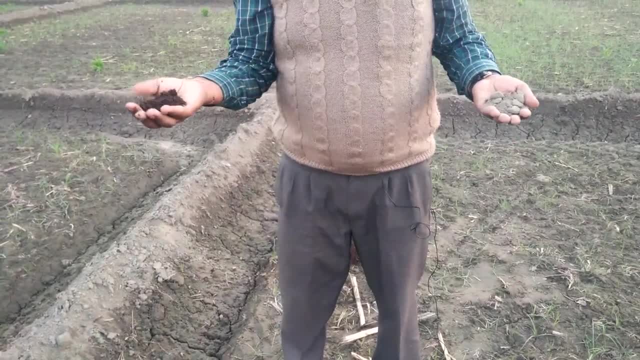 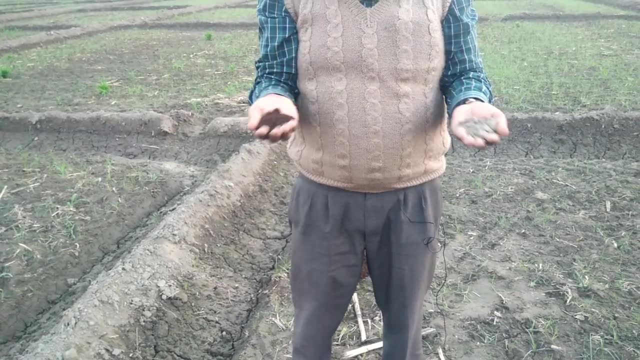 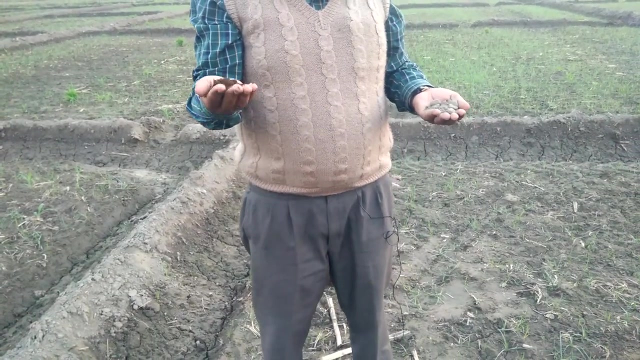 that is being absorbed in this is about four to five times higher. then the water holding capacity, or the absorption capacity, is very high. Similarly, if we look at the CEC- the cation exchange capacity in argumetal and humus, the CEC is about 152 to 300 centimoles per kg of soil and in this soil 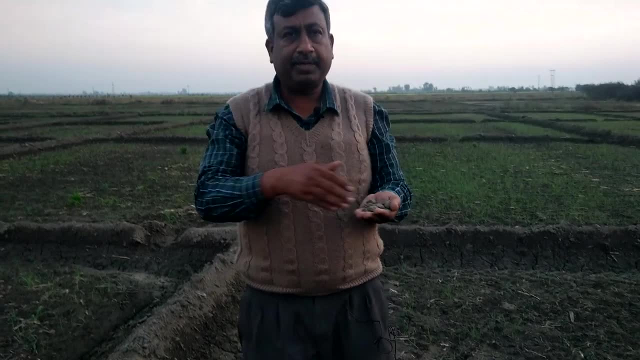 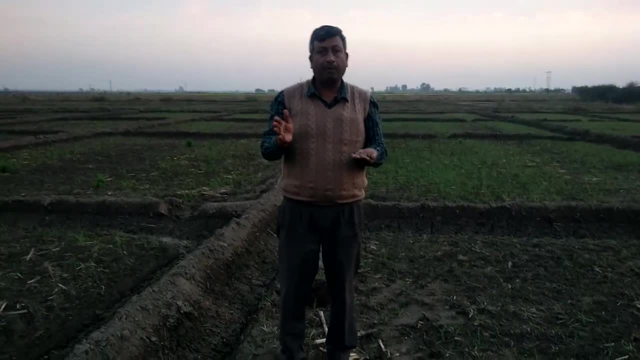 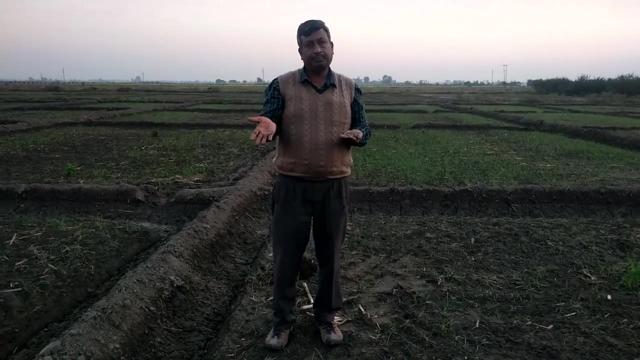 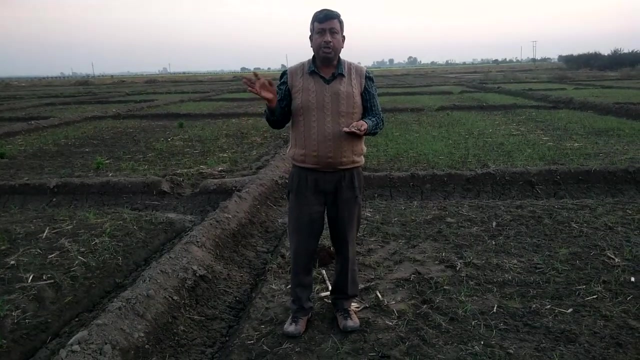 centimoles per kg soil. it means it is just half of humus. and if we take calonite, it is about 3 to 10 centimoles and elite it is about 10 to 30 centimoles per kg soil. Now we can see how much CEC is present in humus and CEC. 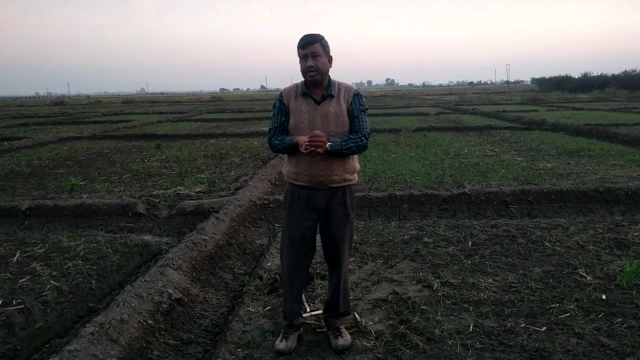 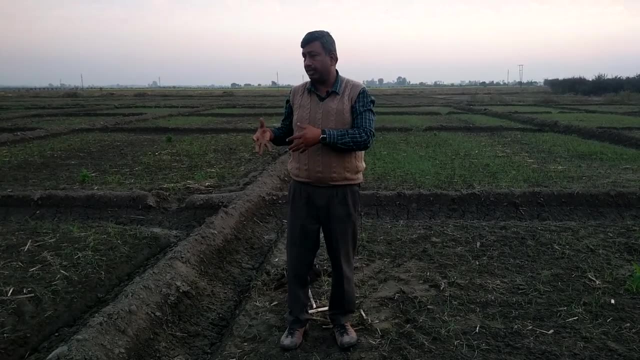 as I have told you many times, has a great role in soil fertility. If there is no CEC, then the cation will never be able to produce humus Because it will be tightly absorbed. So this means that it is an argumetal soil, so it definitely has more CEC. 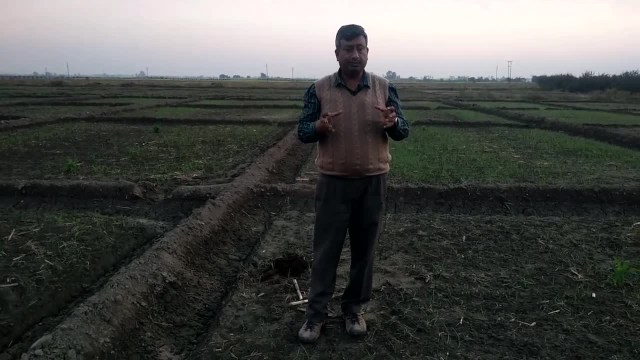 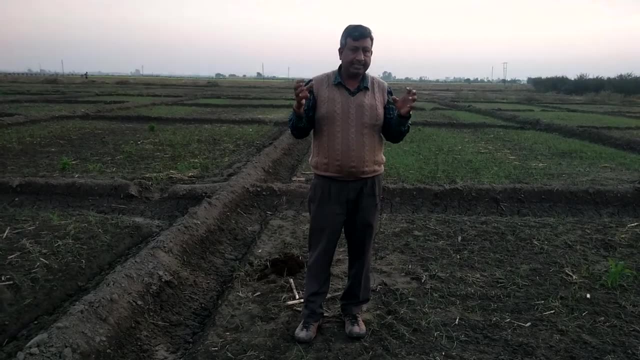 So I told you that humus contains humic acids, and humic acids react with the minerals and extract their bases. Because it is an acid, it will react with the bases in the minerals and that's why extract the bases, like potassium, calcium, etc. 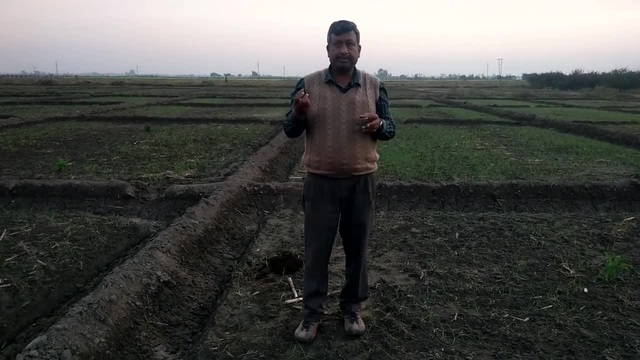 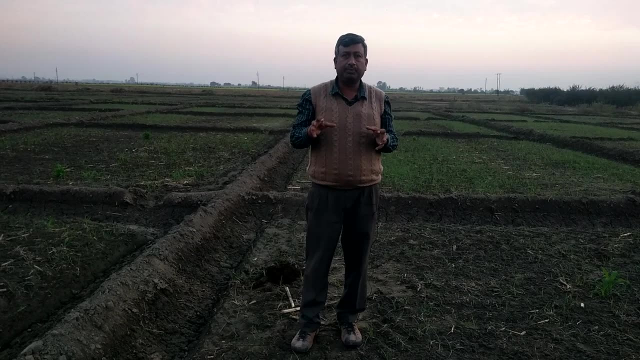 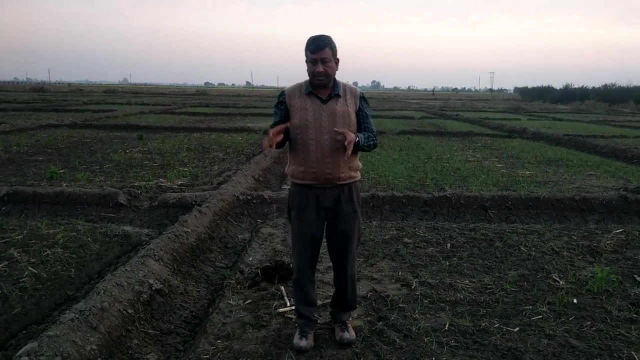 So what will happen? in this way that the nutrients in the clay or minerals basis of inequality? where will they come? Soil solution will YG and also DEா-degraded products, like humus, whether they are nucleic acid or a protein, that are present in soil and these are very beneficial for plants. 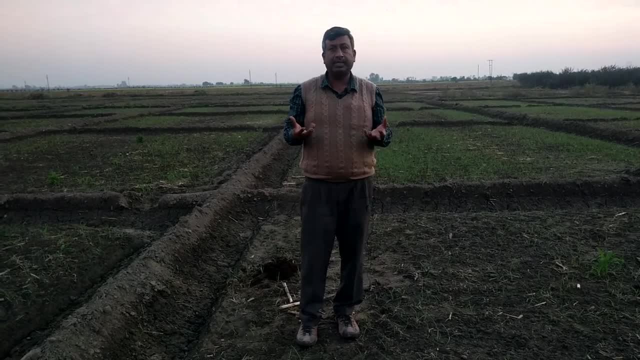 So subscribers? humic acids as such is beneficial for plants. This has been participated in research. Humic acid also has beneficial effect. It means that there is an argumeter: definitely there will be humus in few number of times. So what we add to the ratio of plants, of argumeters to plums or regimens Pour plants, when we include plant, which we do in the리 cases, plants get similarity. but anybody from certain time will get the same difference by how much we Invest inаюgumeter non vezes diu na. 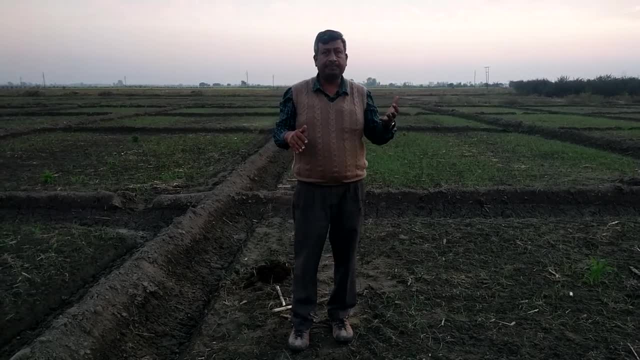 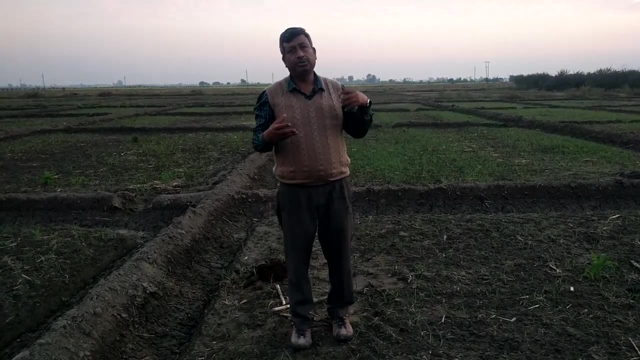 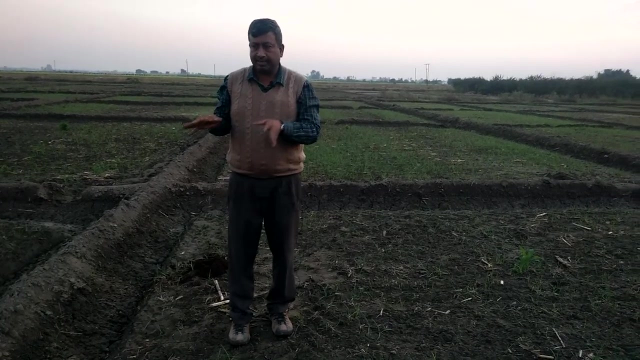 So after we see after one year, if we see what happened to the plant residue after one year, two-thirds are lost as a CO2, two-thirds go into CO2 gas and one-third remain in soil. One-third will remain- 30% to 35%- and 5% will remain in microbial tissue, microbial cells. 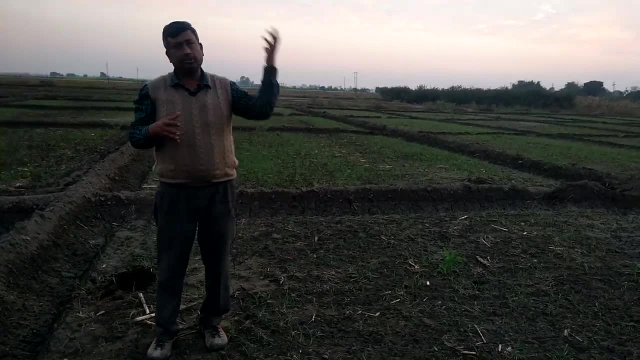 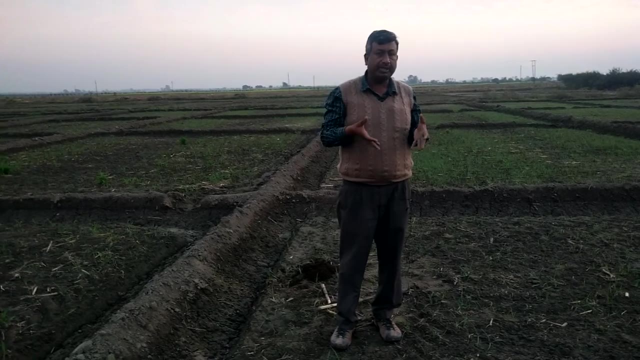 So this means that no problem, one-third or two-thirds will go into CO2, one-third or one-third will keep forming. So what will happen? Humus will develop and then our soil fertility will improve, But if we are not adding organic matter, then what will happen? 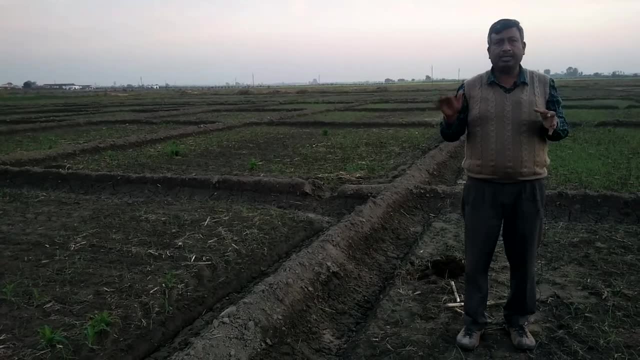 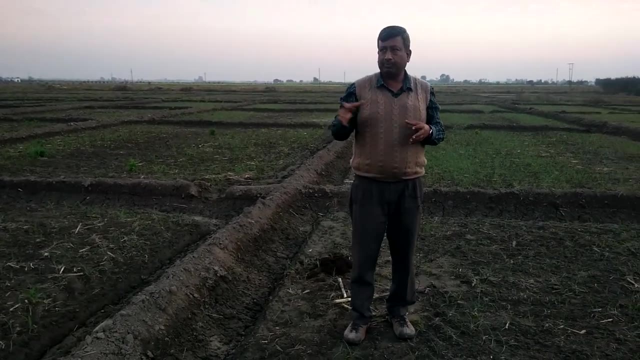 Gradually, the organic matter that was present- one-third- will gradually decrease because microlaction is taking place and there will be a loss of CO2.. So it is important that if we want to maintain soil fertility, then every year we have to add organic matter. 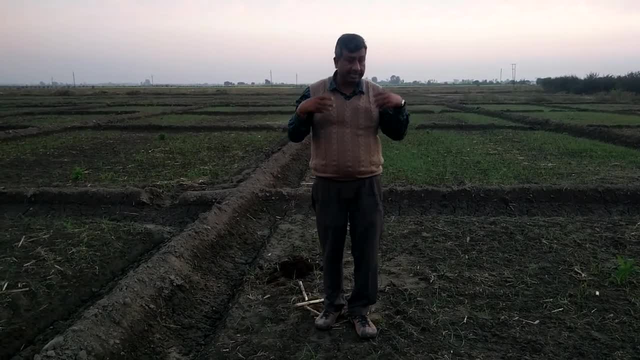 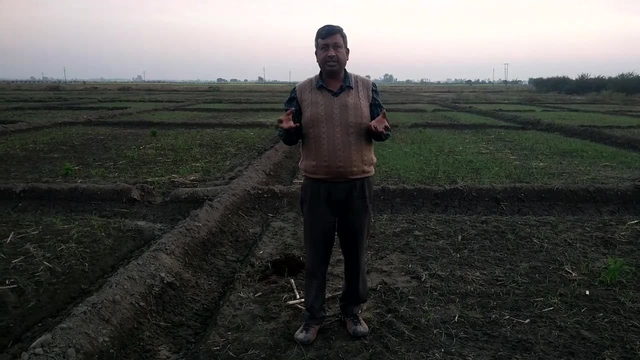 So once humus is formed, I told you that it is highly resistant, so its decomposition will not happen. So what will happen? It will remain as such. So now, if it remains as such, then what will happen? Because it will not release nutrients, there will be no decomposition. 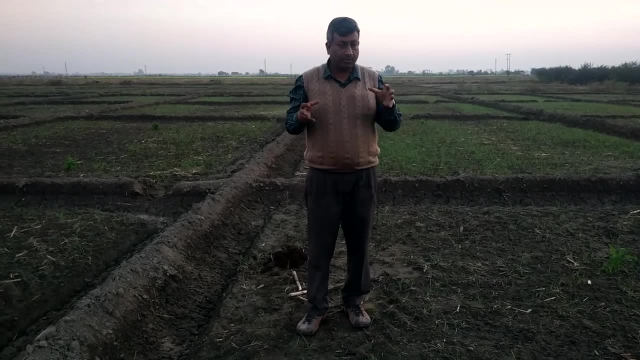 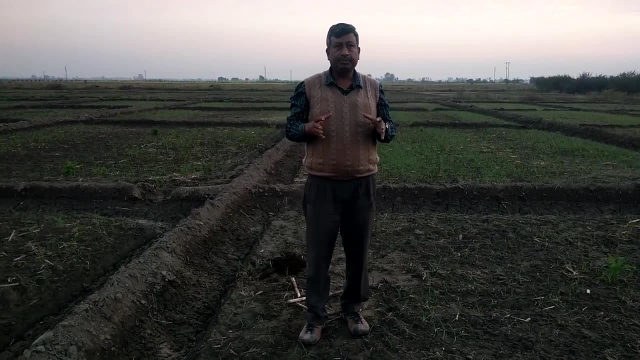 The advantage is that it has very high water holding capacity- aggregation. So water holding capacity will be maintained. porosity will be maintained. there will be aggregation. This is the advantage. So once humus is formed, it is not easily lost. 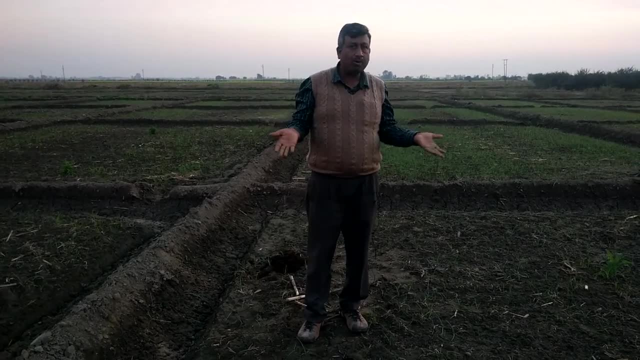 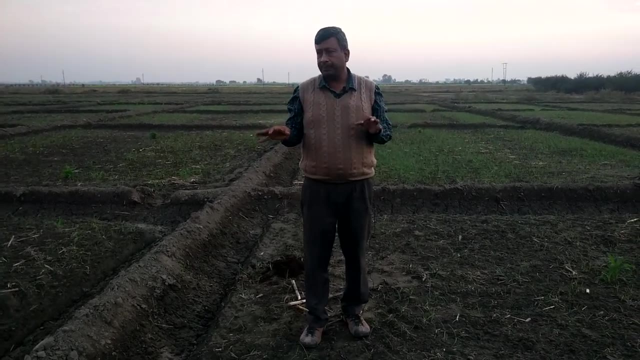 So now this does not happen. So the humus that will be made in this soil, it will be made 100 years ago, it will be made thousands of years ago And it does not lose so quickly. It takes time to be formed and the loss is conveyed. 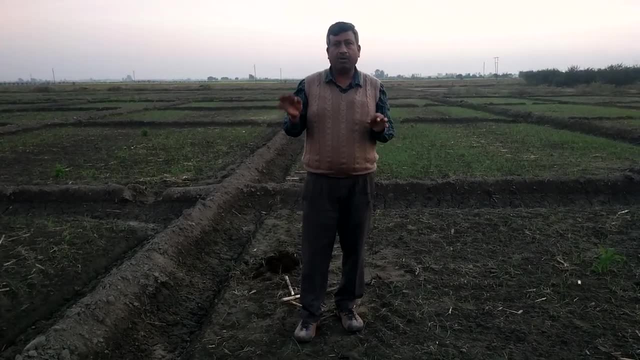 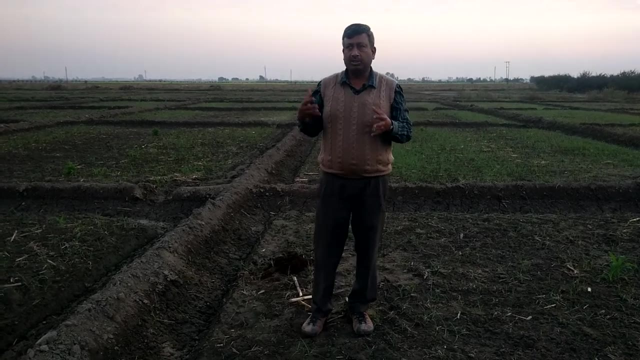 That is why it is suggested that add organic matter every year. So I told you how humus is made from organic matter and how organic matter is beneficial for soil. So if we categorize it and see on physical properties, chemical properties and biological properties, 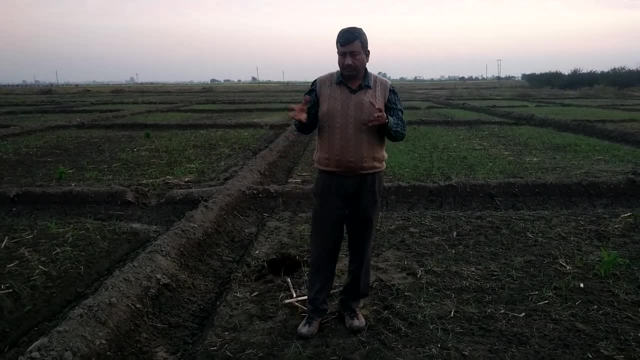 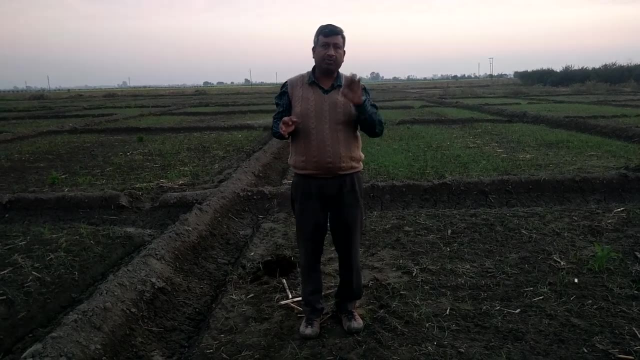 So number one is physical property, Since it helps in aggregation, because I told you there are polysaccharides. What do polysaccharides do? They help in aggregation. Then, coating of humus around this clay particle helps in aggregation. 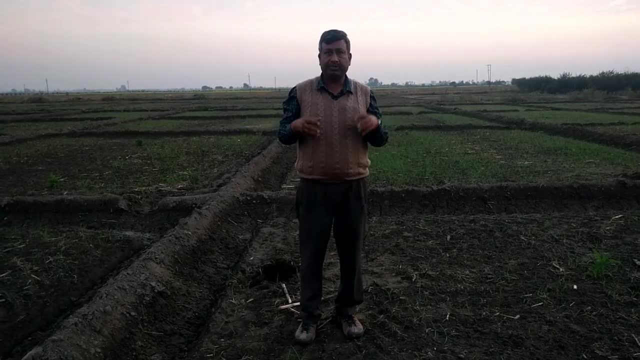 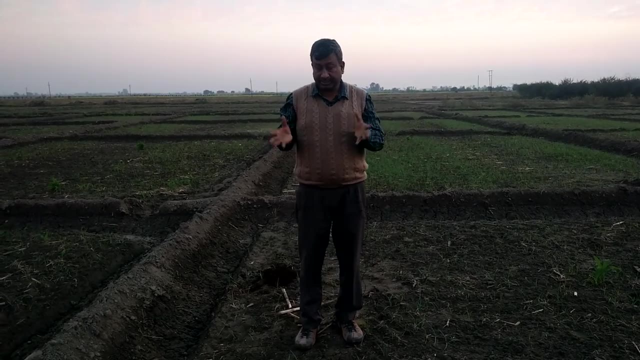 Fungal hyphae helps in aggregation And because of this aggregation, porosity is maintained. infiltration is there, proper percolation is there. So what will happen with this is that the porosity of this soil will be maintained And it is necessary to have a definite amount of this pore. 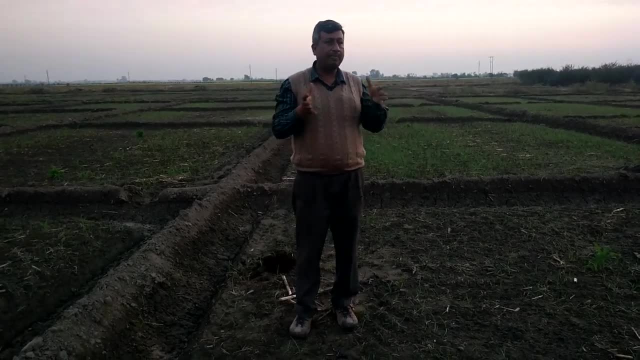 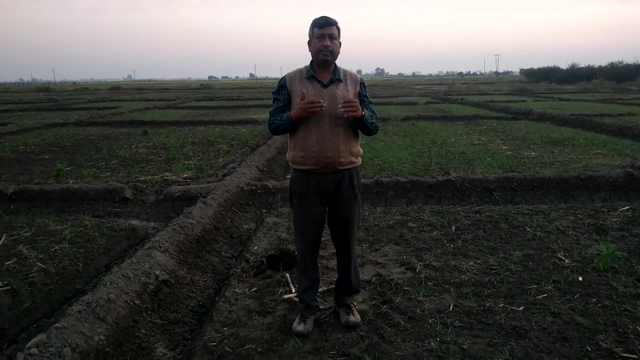 So whether the pores are very high or very low Now, in sandy soils, macropores are very high. In clay, micropores are high. When we add this organic matter, it will maintain the porosity. It will keep a proper ratio of macropore and micropore. 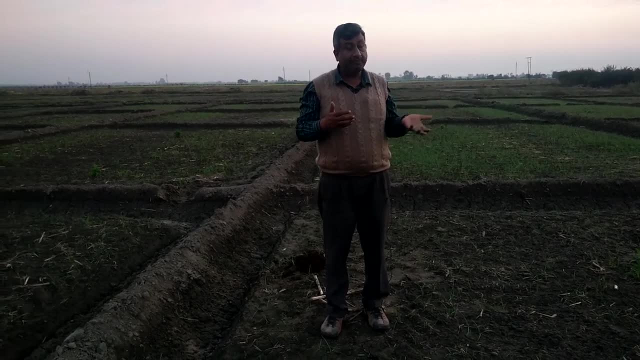 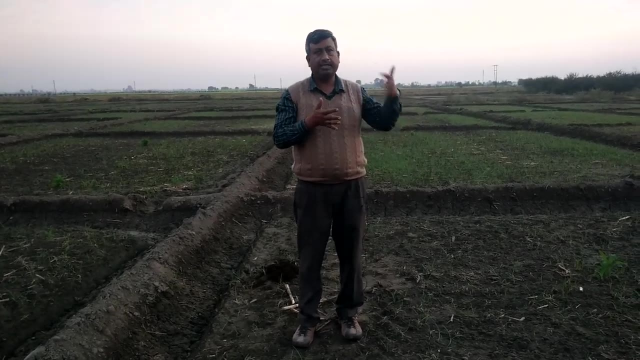 Macropores are essential And helpful for air circulation and micropore for water retention. So when we add this organic matter in clay soil, there will definitely be a reduction of macropores, And when we add it in clay soil, there will be a reduction of micropore. 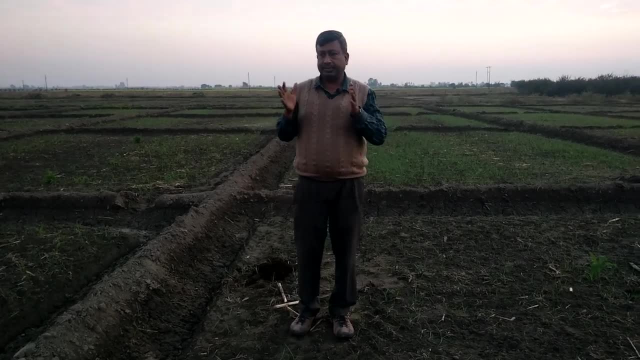 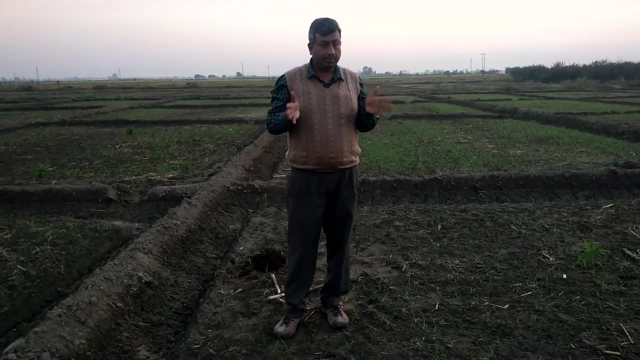 So it will bring both of them in a balanced situation. So this will help in aggregation, percolation, infiltration. Root proliferation will be good. Then bud density is reduced. It will reduce bud density. Bud density is a very important factor which decides the root growth. 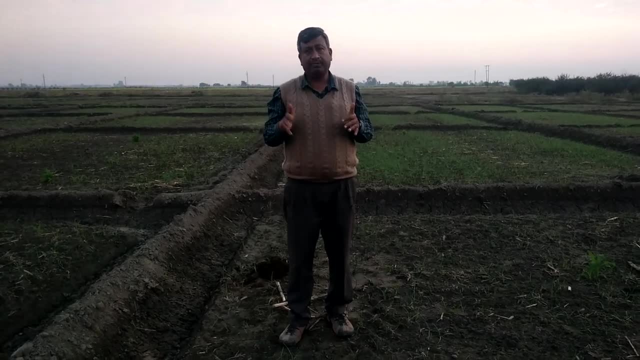 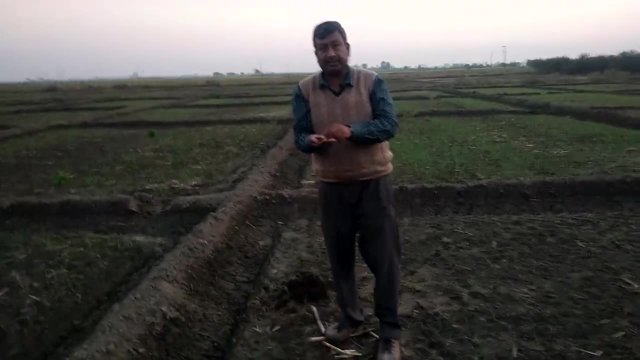 And aeration and water retention. So generally this is a very light material. It is very light And you can see the color: It is dark brown. So when we add this in clay soil, the weight of the soil will also be less per unit volume. 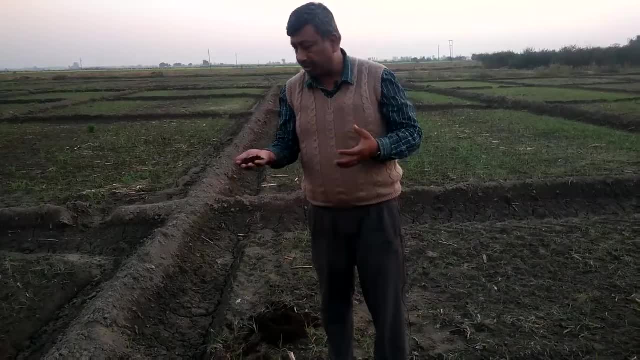 So its bud density will be around 0.3, 0.4, 0.5.. And the normal bud density of soil is 1.3, 1.4.. The bud density is this much, So when we add this in clay soil, the bud density is reduced. 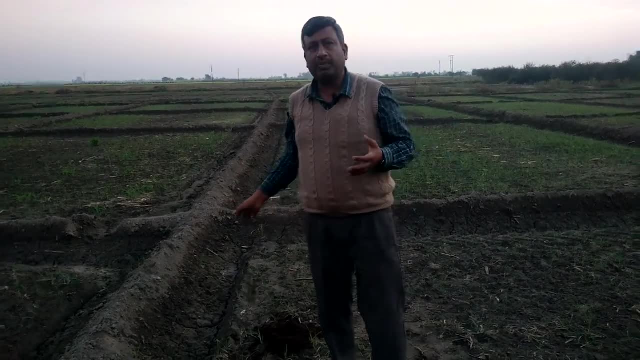 Bud density is reduced means there is proper porosity, Proper root growth. So this is a very important factor. So when we add this in clay soil, there will definitely be a reduction of macropores, And when we add this in clay soil, there will definitely be a reduction of macropores. 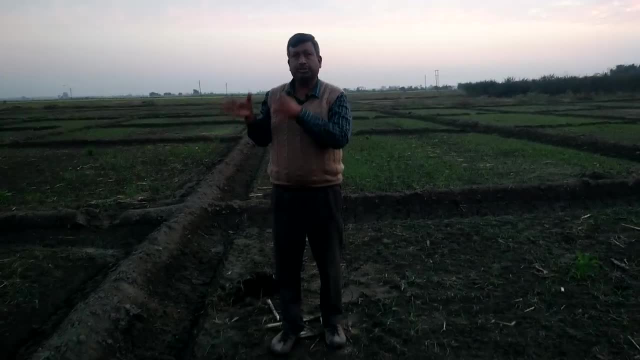 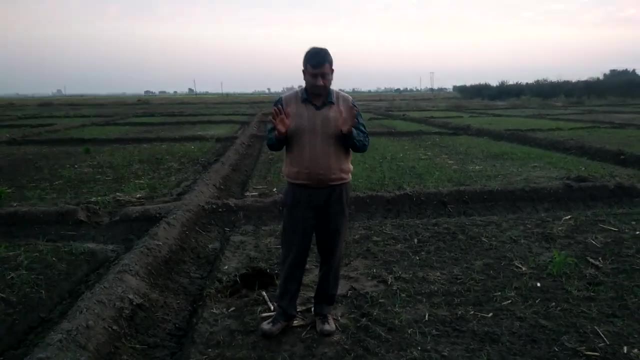 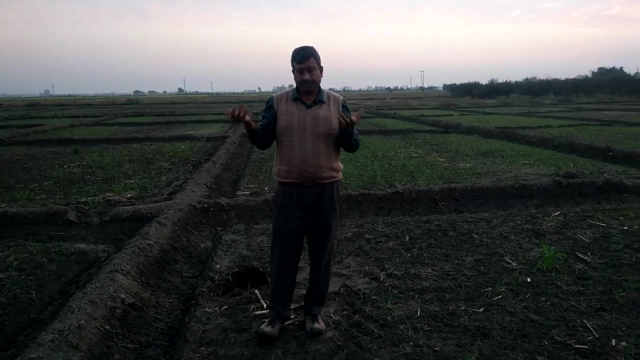 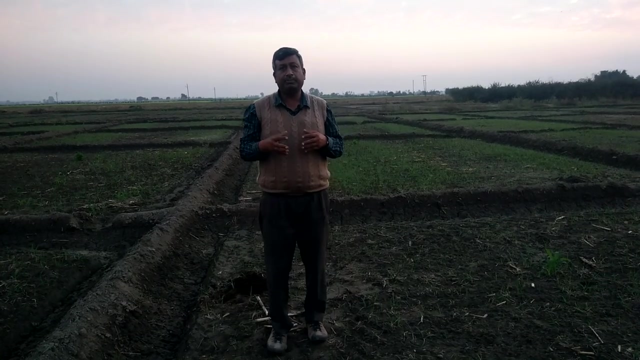 So this is a very important factor. There is one last important thing you need to remember If you see the chemical properties. number one: it helps in enrichment in nutrient because during decomposition nutrients are released. And how do nutrients release? I will give you a complete lecture about that later. 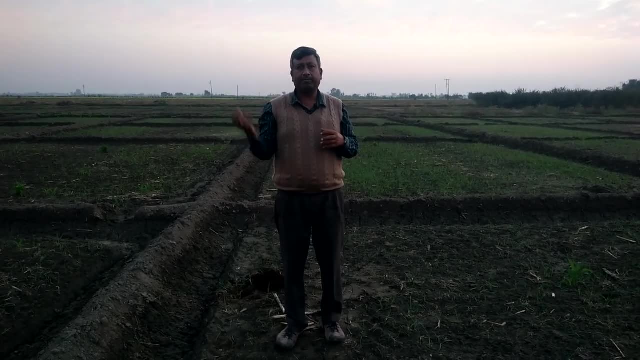 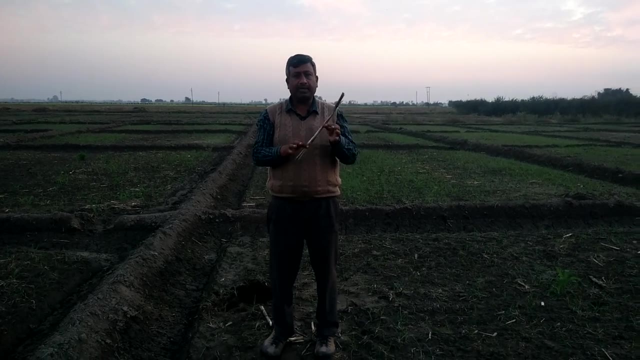 But now let us talk about the ole wrench. I will tell you how the decomposition takes place and how the nutrients are released. So in this there is N? P, K, Sulphur, Calcium, Magnesium. all are present and during the decomposition, 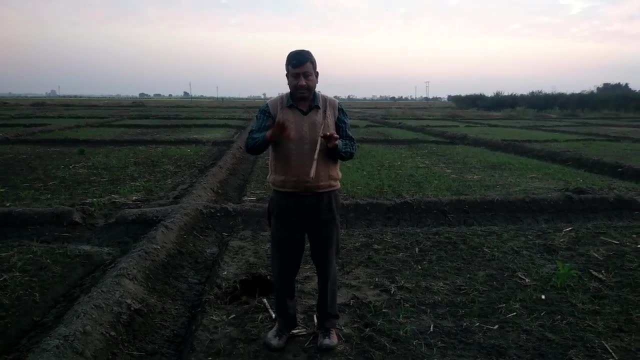 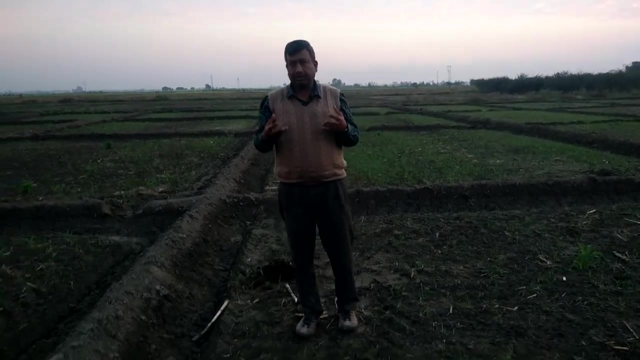 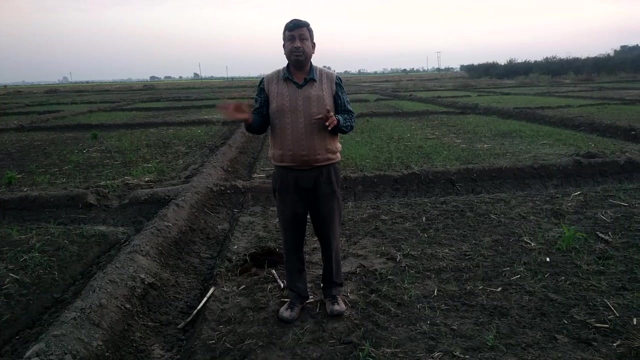 these nutrients are released and now, after the release, they come into soil solution. So what will happen to the soil? Fertility will be enriched. So during decomposition, several nutrients are released and there is a pool of nutrients. Then second, CEC, high CEC. about 30 to 70% CEC is contributed by organic matter. 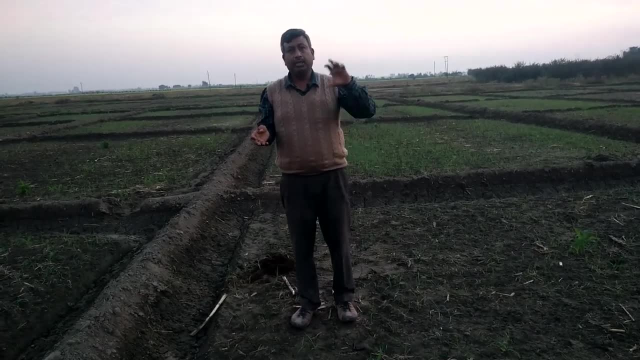 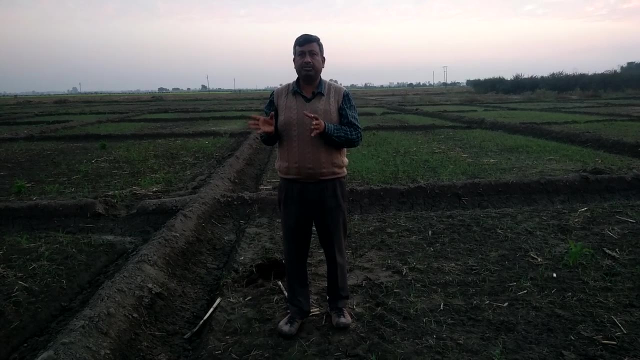 Now I have also told you its value: 150 to 370 mol. How much capacity is it doing? But if we take out the total soil, CEC, about 30 to 70% CEC is contributed by organic matter. And what will happen if CEC is more? 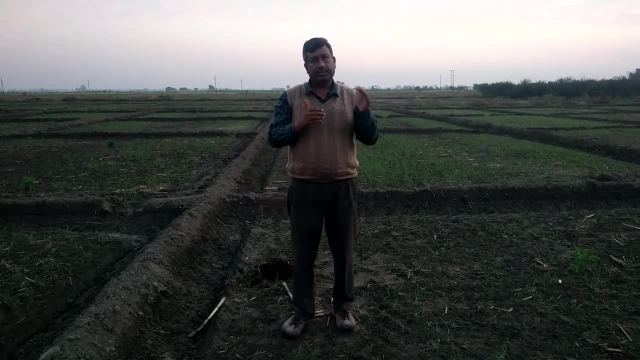 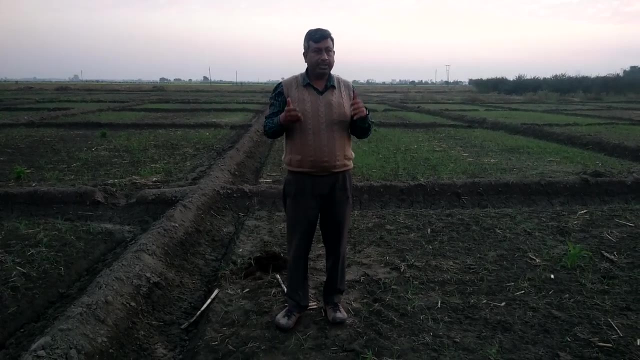 The nutrient will be exchanged between the solid particle to soil solution phase, and then plant can easily absorb. So this is its advantage. Then nutrients: Nutrients are present in organic matter, and 95 to 99% nitrogen is contributed by this organic matter. 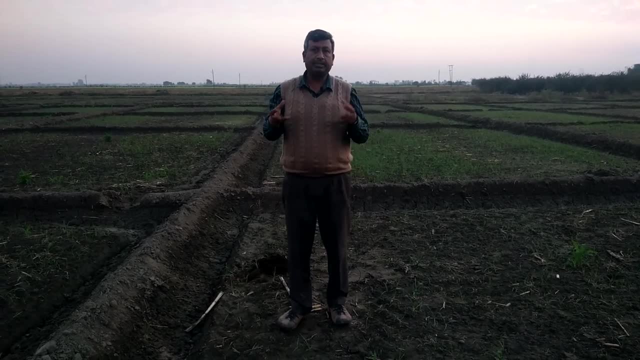 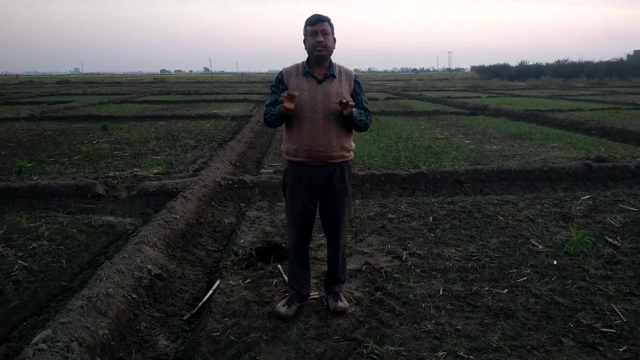 And about 75% Sulphur and about 33 to 67% Phosphorus. So I will tell you in detail how the decomposition happens and how the nutrients are released. But now in this lecture you have understood that organic matter releases the nutrients after decomposition. 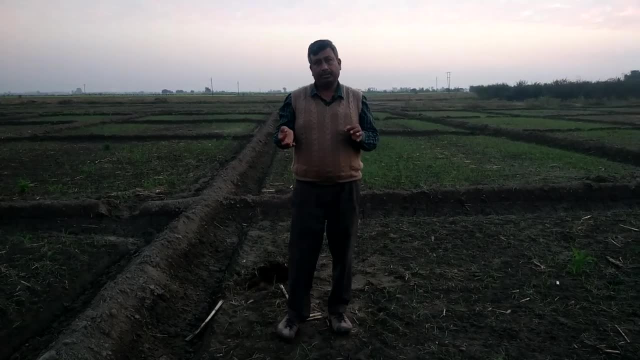 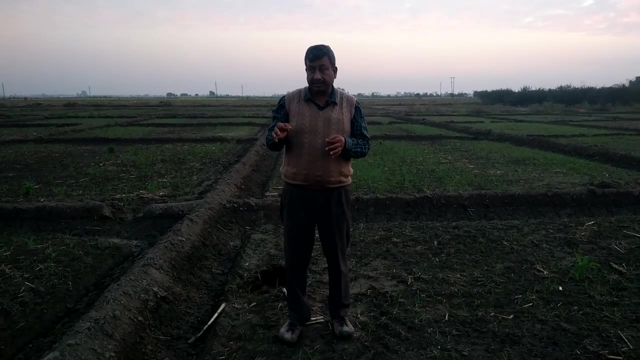 and these nutrients are absorbed by plant. So this is helping in chemical properties by CEC And these charges. and this CEC is due to charges, As I told you: hydroxy group, phenolic group, carboxylic group, 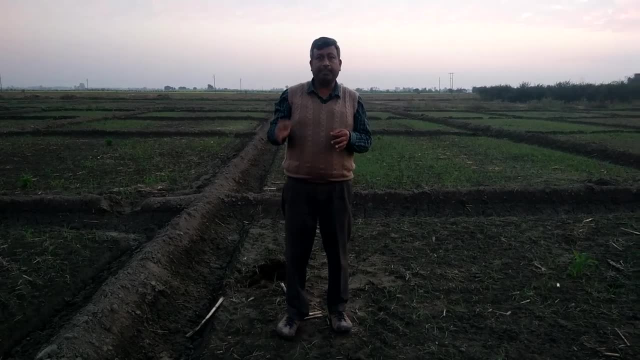 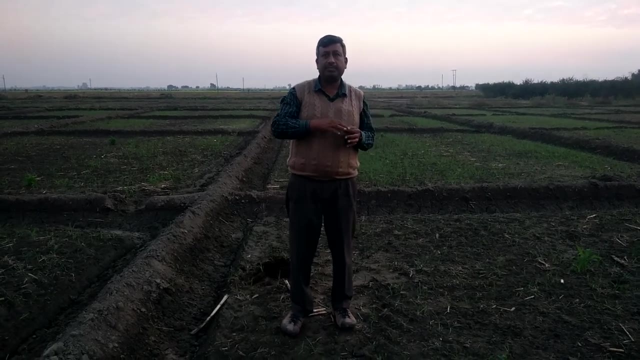 And these negative charges are pH dependent. So as soon as pH decreases, acidic soil is created, its charges will decrease Because they are satisfied with it. they become hydrogen ions. But as the pH is increased, CEC is increased. So CEC is very high and soil fertility will be improved only by CEC. 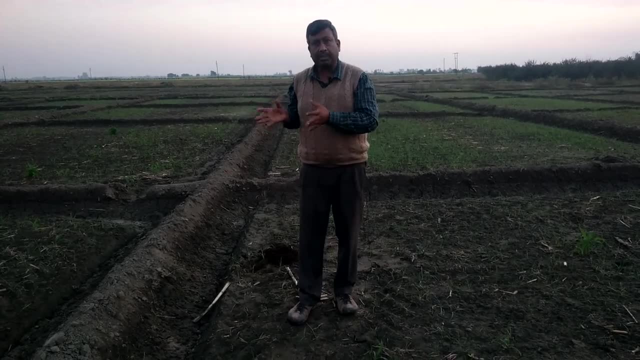 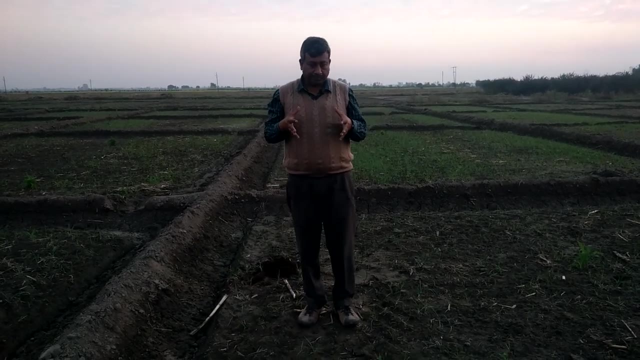 So as a source, as a reserve of nutrients, it is working as a reserve. It is supplying nutrients, It is holding nutrients And it makes the complex with the micronutrients. Now see organic matter which is made of metal complex. it helps a lot in this. 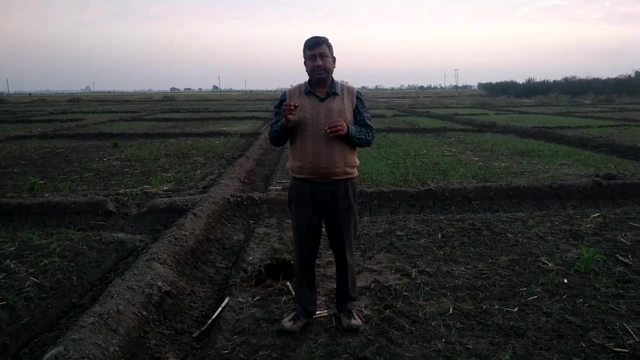 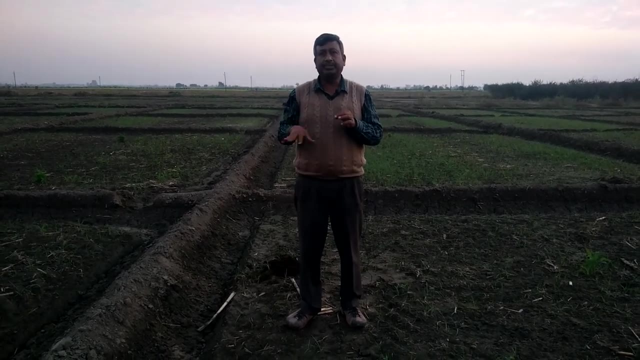 The zinc, copper, manganese. it makes the complex and prevents the leaching And after a few times it releases these nutrients. Otherwise, if there is no complex, then these metal nutrients may leach down. So the organic matter which is being made, the organic mineral complex which is being made, 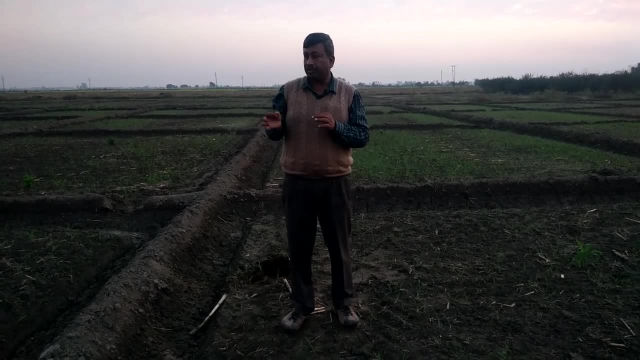 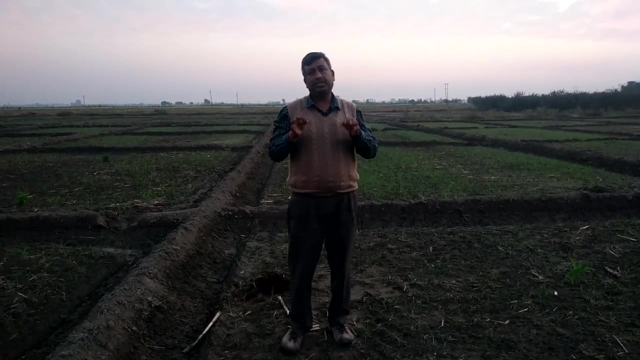 that is beneficial for plant. But if there is too much organic matter, if it becomes too complex, then it will not be released. So too much organic matter should not be added, Otherwise the chelates of the micronutrients will become very strong and these chelates will not release. 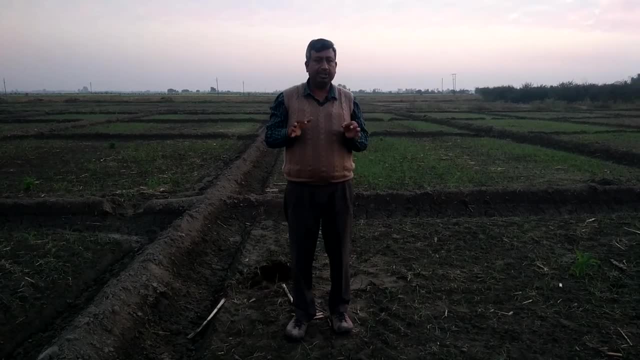 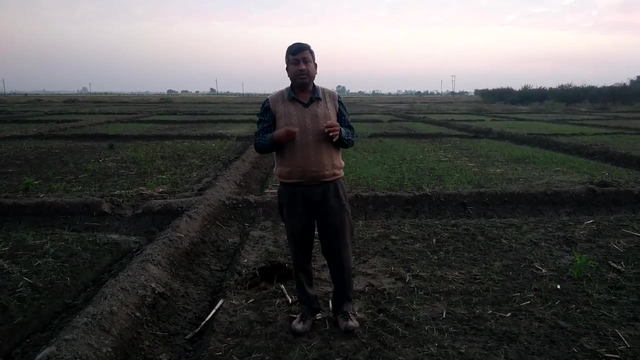 So the chelate in a definite quantity is beneficial, But it is not beneficial in a huge quantity. So I told you about the chemical properties. Then humic acids are released, And this humic acid is helpful in reducing alkalinity. 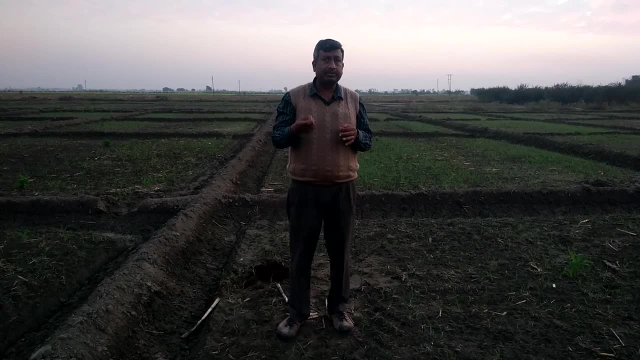 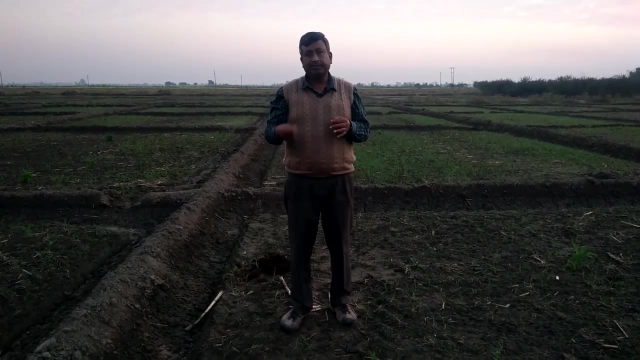 So there is alkaline soil and saline soil. If we add organic matter in that, then during decomposition definitely organic acids are released, Humic acids are released And these organic acids react with the salt and reduce the alkalinity. Thus reduces easy electrical conductivity of soil. 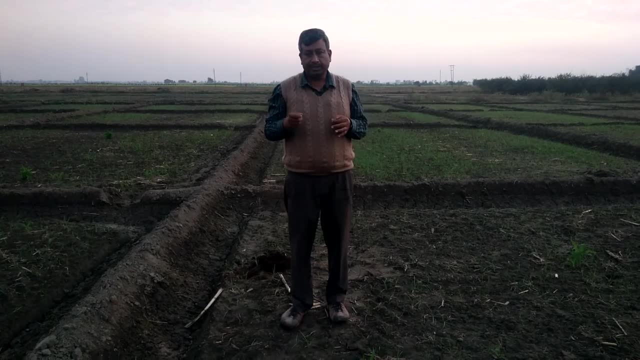 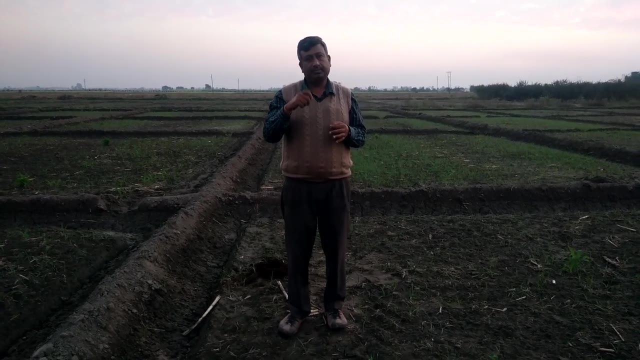 So see, this is also helpful in saline and alkaline soil, And then in acidic soil it reduces the toxicity of aluminium. So this is beneficial in both the soils, In acidic soil also, and in saline and alkaline soil. Now see the biological properties. 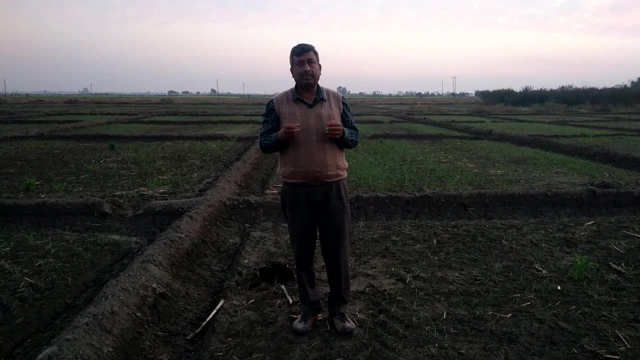 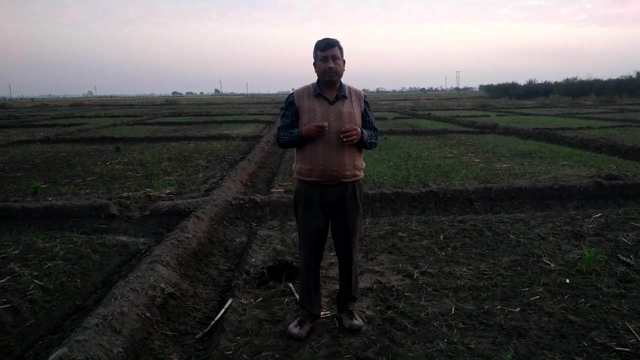 Since it has carbon, and carbon is food source. So when we apply the organic matter, there is a huge increase in population of microbes because they use the carbon. So look here: When we will add the calcium, what will happen in this soil?